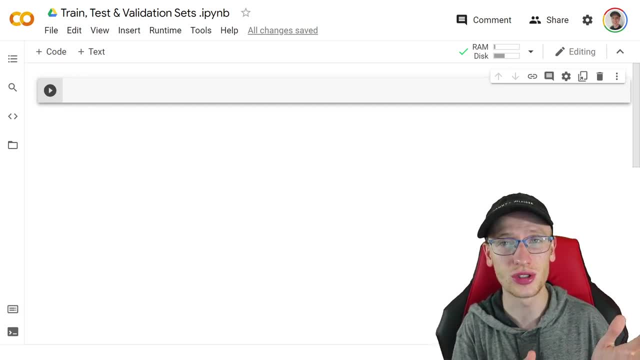 your skill level is whether you're just touching machine learning, you're just googled these terms or you just ran into this. it is going to be a really helpful video for you. So the main idea that's important for now: to run a machine learning model, it needs to be trained on data And we also 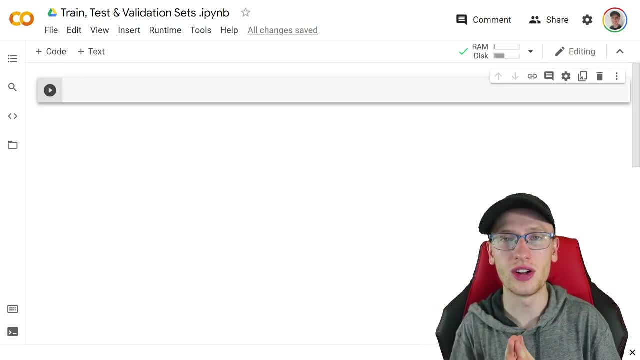 don't need to just train that model. we need to evaluate it on data to know that it's actually going to perform well. So we definitely have two splits or partitions of a big data set. We definitely split it into a training set where we train the model on that data and then we test it. 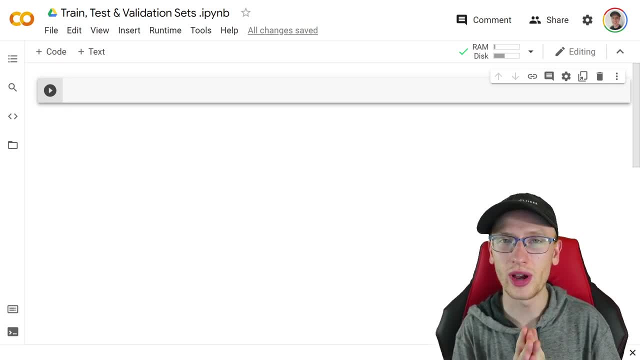 and evaluate that. But in this video I'm going to show you why you actually need a third split of the data. but we're not there yet. For now, we're going to assume just that approach of train and test and we're going to run into a problem and we're going to see why we need that third. 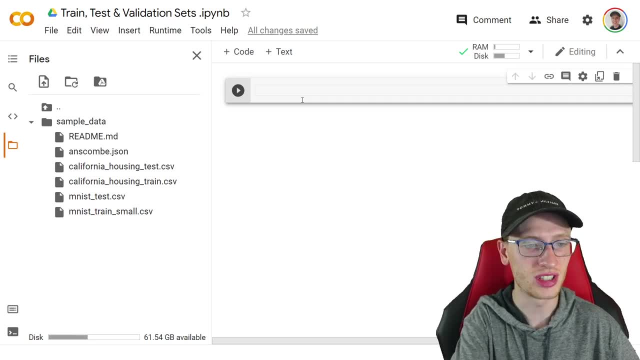 split. So the data set that we're going to use is California Housing, and you can see that there is a lot of data set that we're going to use. So we're going to run into a problem and we're going to test and train here. We'll train on this and we'll test on this for now. So dftrain. 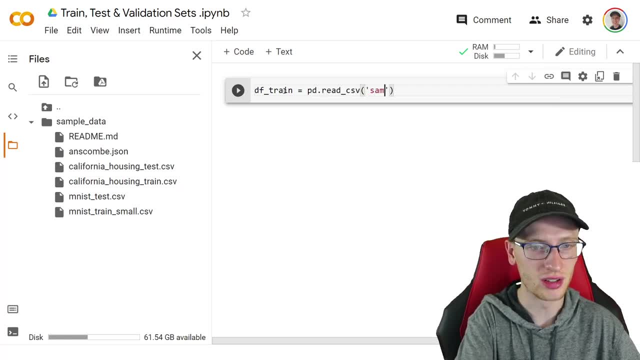 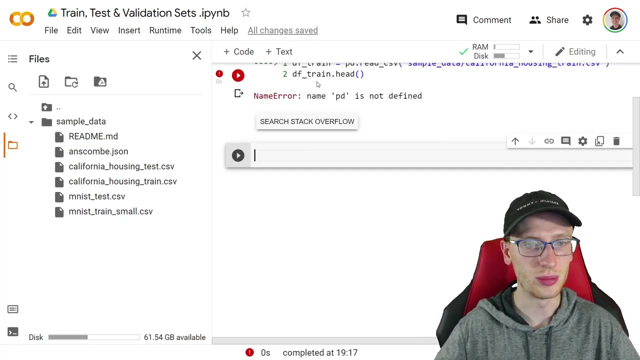 we'll call it is equal to pdreadcsv of sample data slash California Housing traincsv. Okay, and then dftrainhead is going to be not defined because we didn't import pandas. Good, start me. So import pandas as pd. 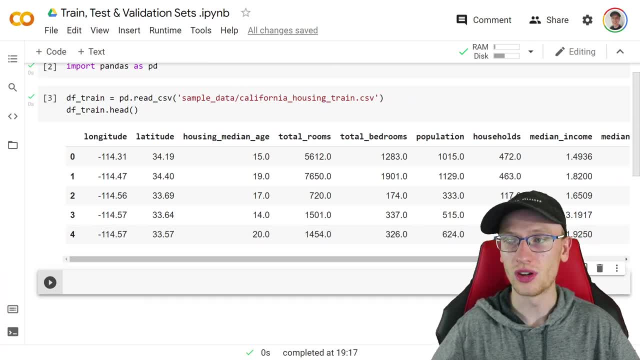 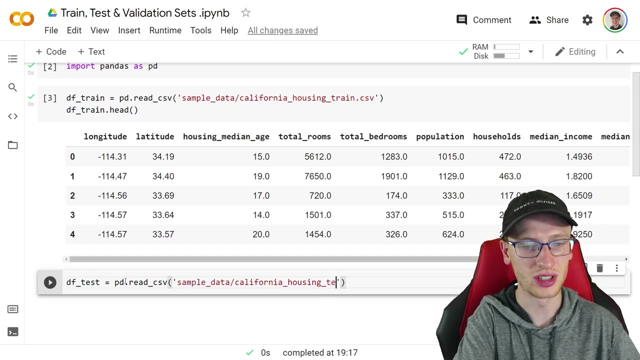 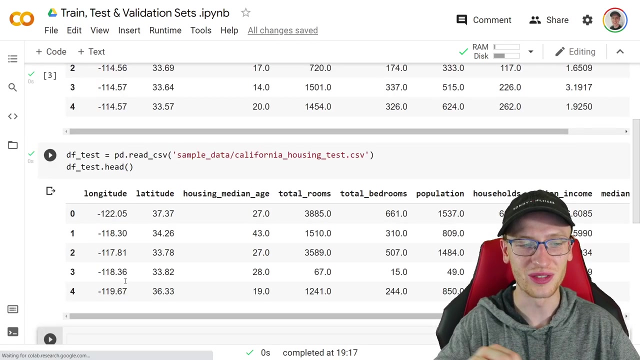 And dftrain. that is our data frame And we can also load in the test data frame very easily with dftest. is equal to pdreadcsv of sample data slash. California- Sorry for this annoying part at the beginning: California Housing testcsv, And we should see dftesthead is like that. Okay. 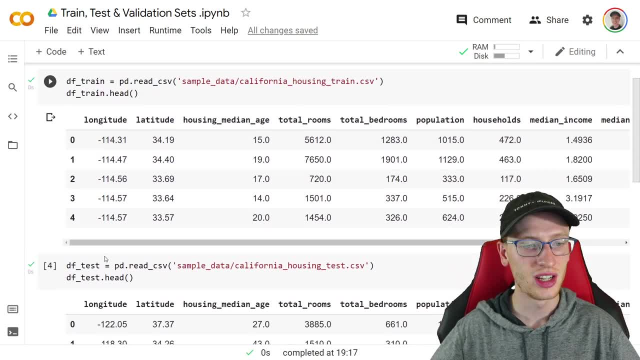 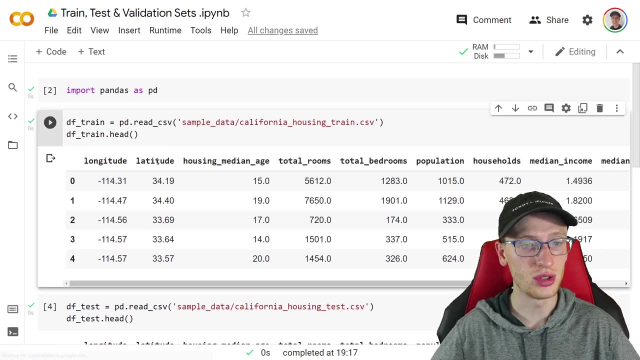 so this is the first five rows of our training data set And these are the first five rows of our testing data sets, And each of the rows of information are all of this: longitude, latitude, housing, median age, total rooms for some area in. 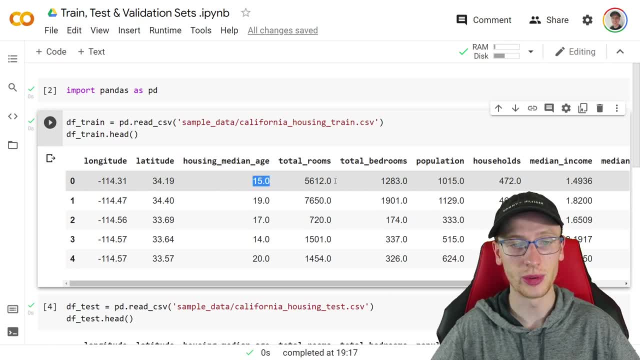 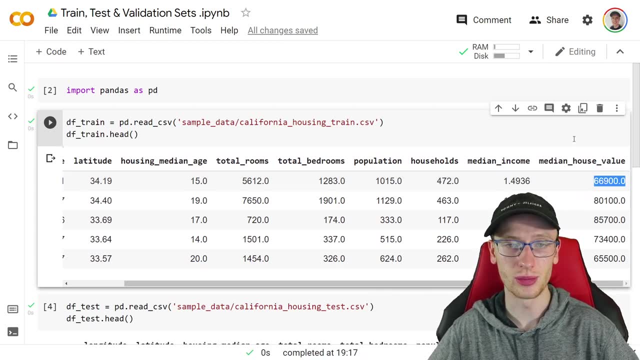 California. So it has some location, It has some information about housing and rooms And the final thing which we're going to try and make a machine learning model for is the median house value. Now I have a full project on this that goes through everything. 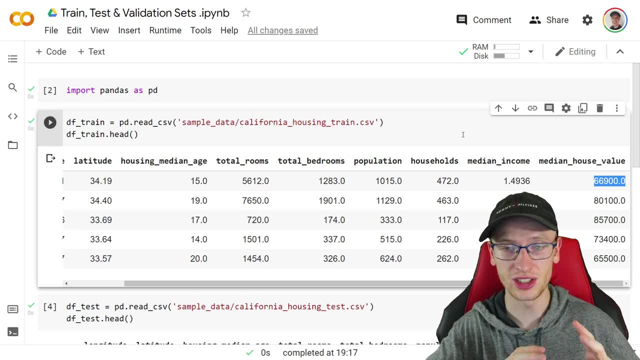 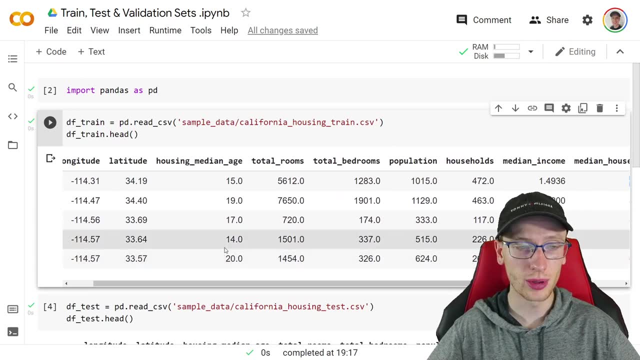 on how to do this. well, But we are going to focus a much smaller, condensed video on the reason for this. So we're going to focus on the reason for this And we're going to focus on the question and how to do it: train tests and validation sets. So, for our purposes, we are 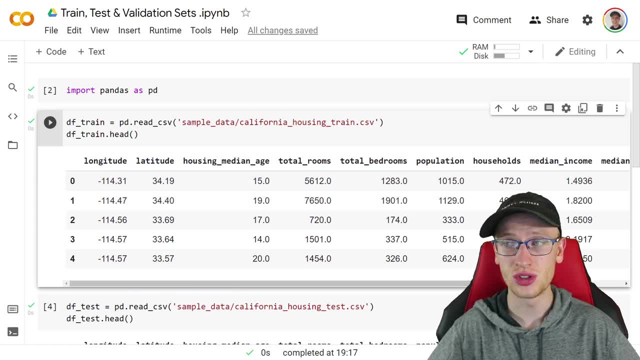 going to just stick to a model or a group of models that use two variables to predict. we're going to use the housing median age and the population- So housing median age and population- to try and predict the median house value. We're assuming there's some sort of pattern. 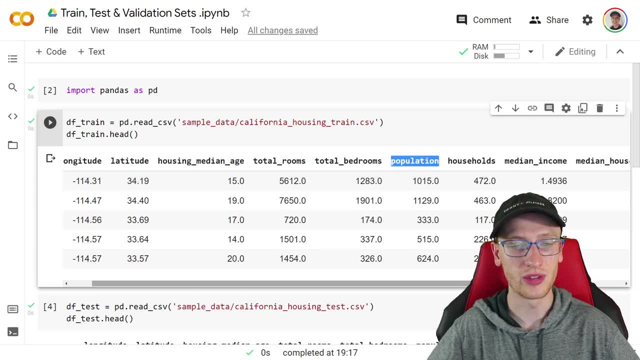 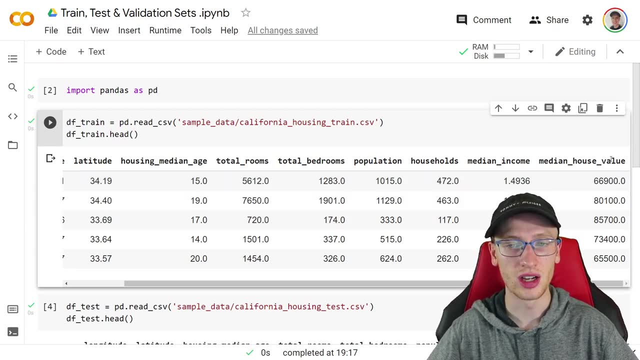 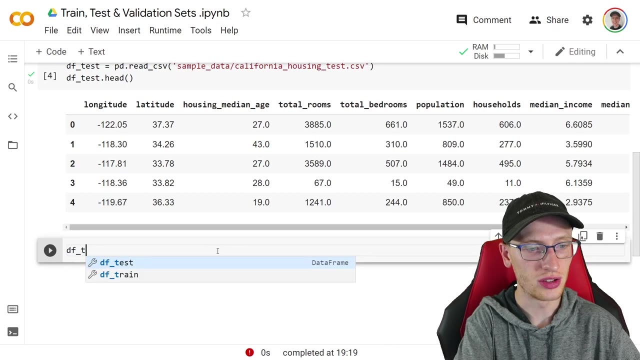 where you can use these variables- housing, median age and population- to try and predict the this continuous value. So this is called a regression problem. we're predicting continuous value of the median house value. Now, since I said we needed those variables, let's go ahead and do tdf train two- I guess is equal to just df train, where we specify we want. 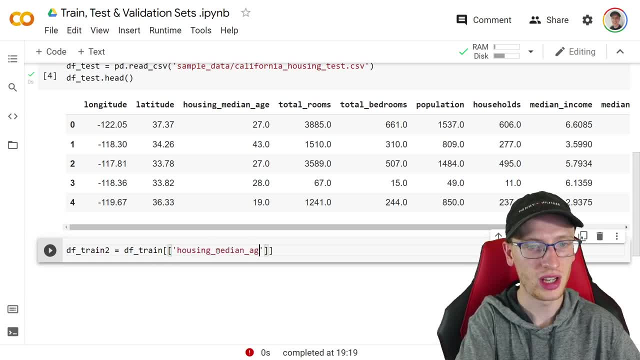 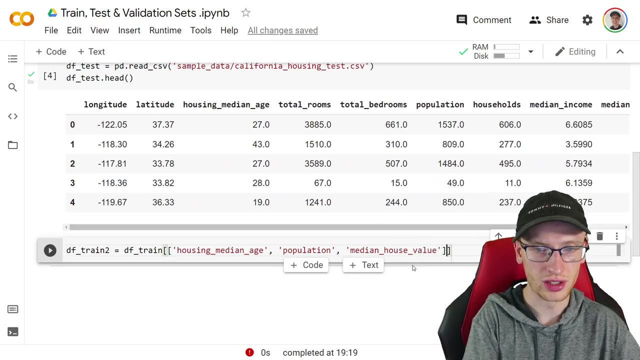 those particular columns, which is housing median age as well as population, And the final one is median as a house, or housing median house value. Okay, so we'll do that And show that the head- the top five rows- is actually. well, there, I forgot to do head. 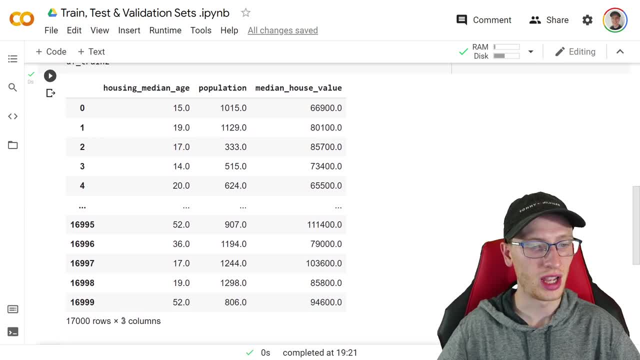 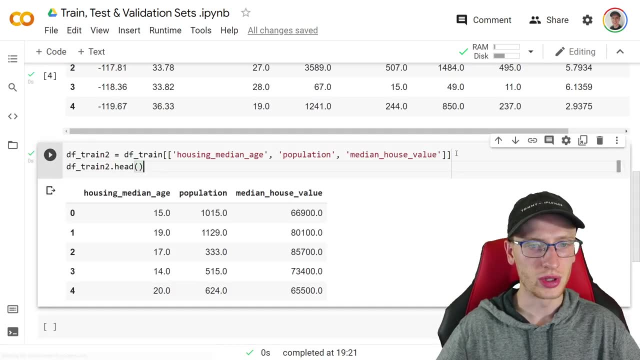 but we have 17,000 rows total- that's actually important to know- and three columns Okay, and just to show the head is right there, Okay, so we will do again kind of a boring thing for now, but the exact same thing. But we are going to switch that to test because we're going to need 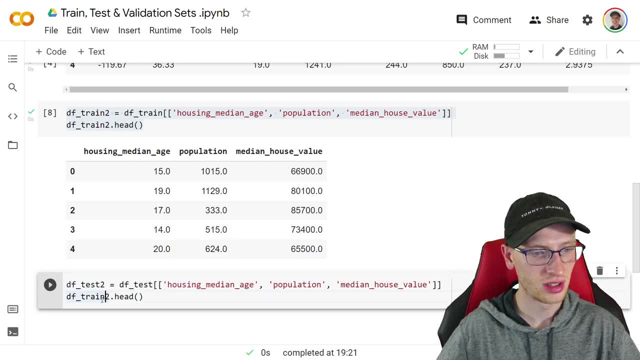 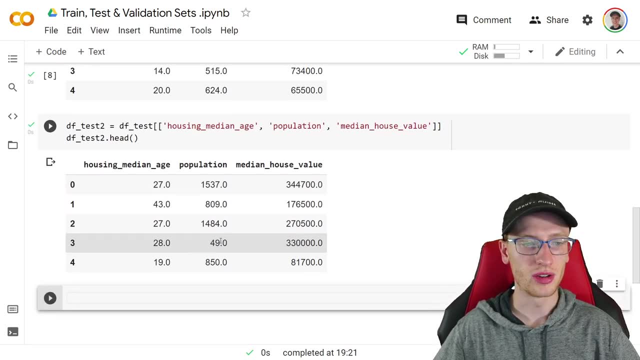 that That'll be test, that will be test, And that will be test. And there we go, Okay. so now that we've got that, let's go ahead and make our first machine learning model on the training sets and then evaluated on the test set. So we do this generally with converting. 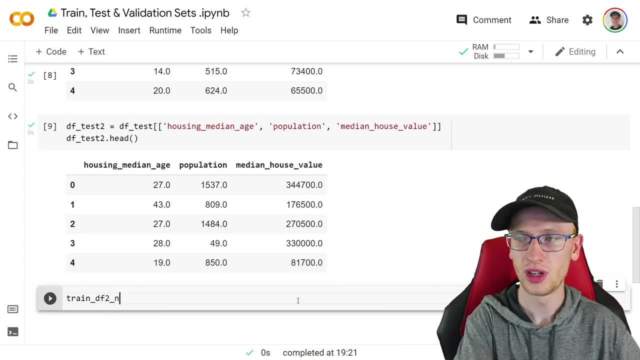 stuff to numpy. we don't have to use too much numpy, So don't worry about it. But we do need to convert them to the data frames, to numpy arrays. So train df to numpy is going to be train df to dot to numpy. That's all you have to do. So that converts that whole thing to this big numpy. 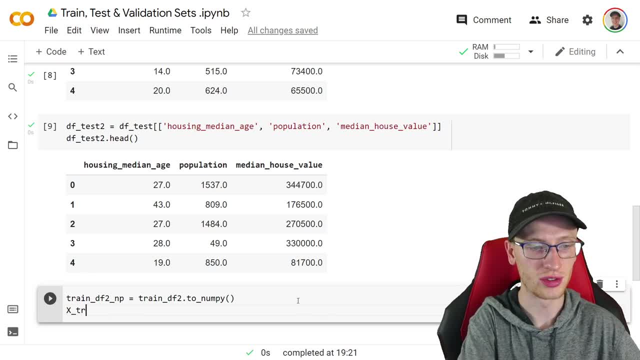 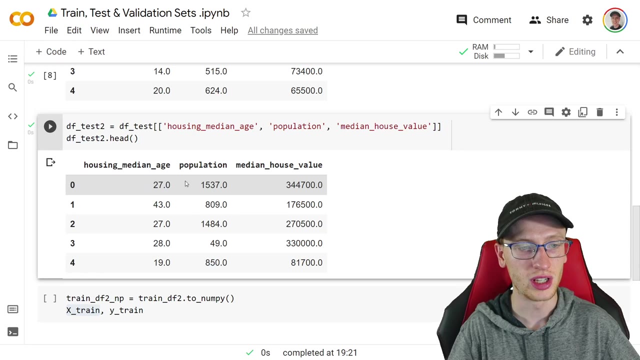 matrix, And then we will take particular columns for x, which is going to be our mark, our input and our output is going to be this y train thing. so how these, how these models all work, is through supervised learning. we feed it. many input, output pairs. the input is going to be, you know, one input is this and that and the output is going to. 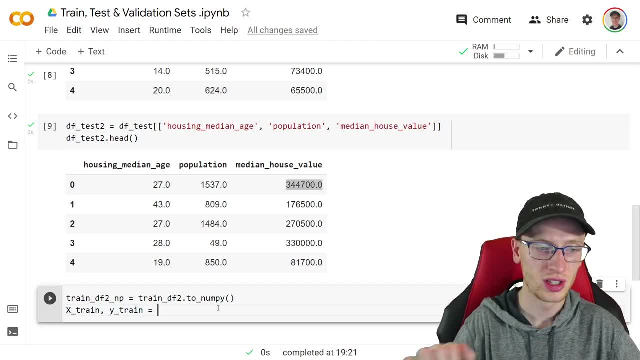 be that. so this is setting up our input and output arrays, where x is this whole matrix of inputs and y is this big long vector of outputs. okay, so x train and y train is equal to train df2- numpy big long name that's going to be. we need to subset of this so we get all of the rows and then the first. 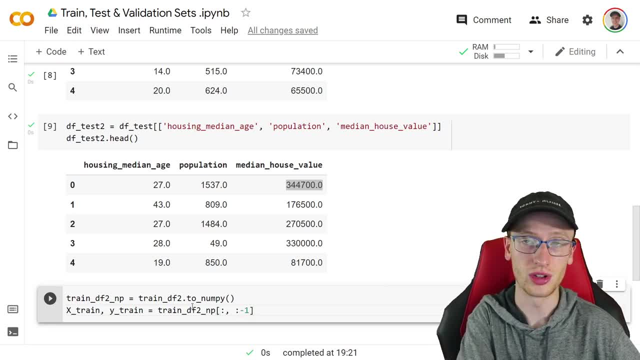 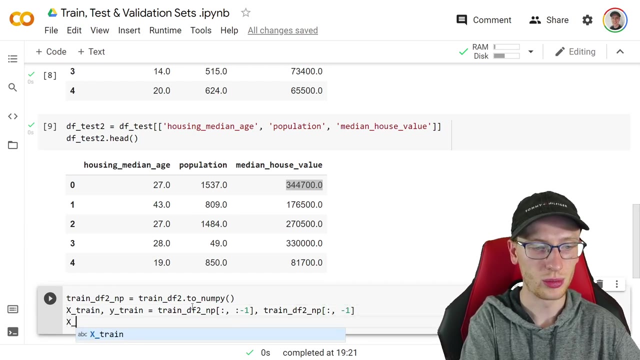 two columns and i can do it like this, where i'm basically saying all, all the columns from the beginning, not the last one, and then train the same thing, train df2 numpy, where we get all the rows and then just the last column, like that, okay, and then we can check their shape, which says how, basically, 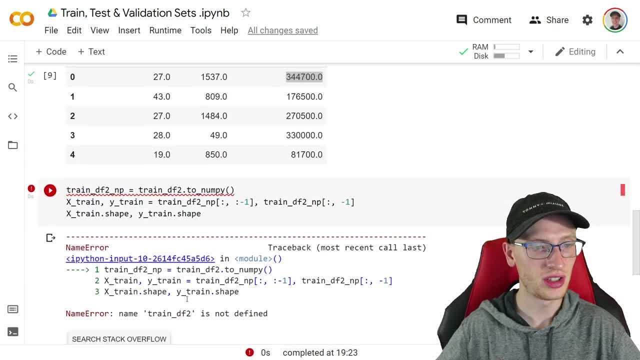 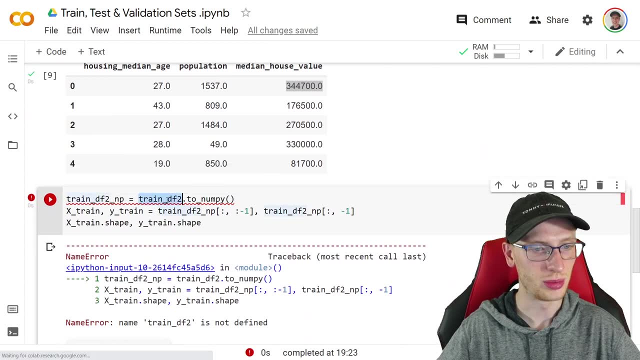 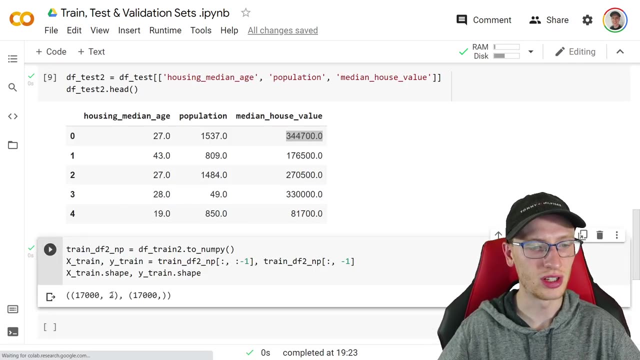 the arrangement of the items and i'll explain that where train df2 numpy train df2 is, does not exist, i must call it something else. yes, this should be. it should be df train, df, train two, uh, two, yeah, two. okay, so 17 000 rows and two columns and 17 000 rows, so that here this is. 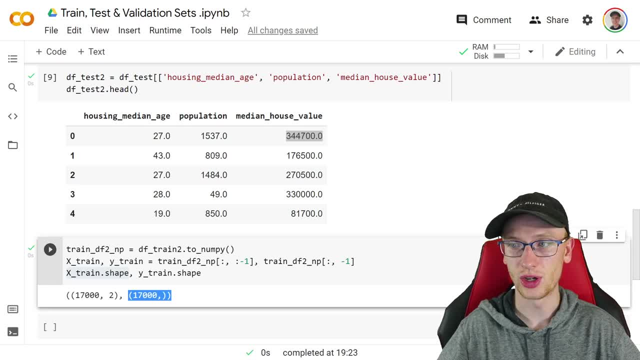 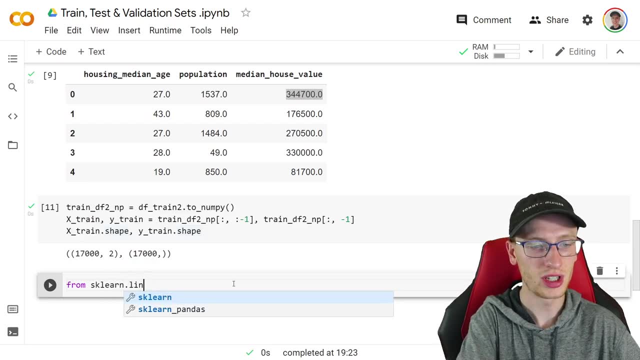 our matrix of input and this is our vector corresponding vector of outputs. we can use this to fit a linear model with from sklearnlinear model import a linear regression. this is just the base linear regression which is going to draw a line through line through data. we will do from: 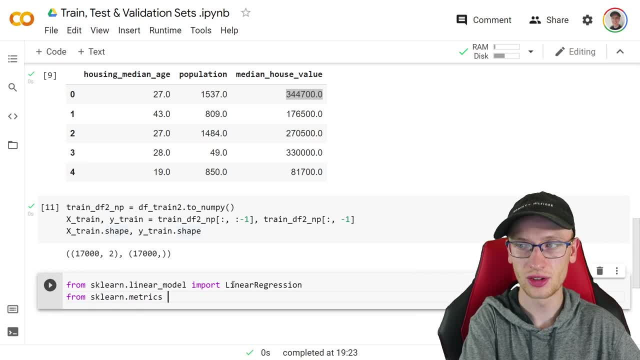 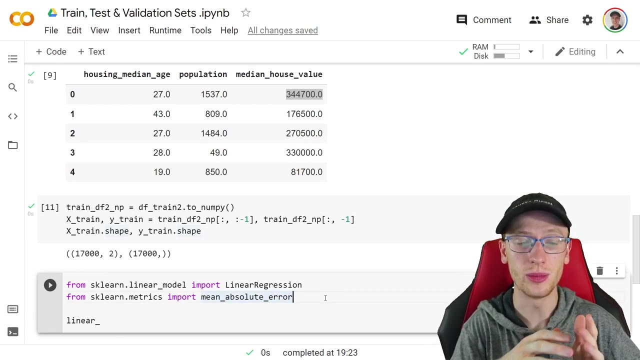 sklearn, sklearnmetrics, we'll import the mean- mean absolute error so that linear model. by the way, mean absolute error is basically just a different measurement. normally we use the average sum of squared errors, the mean squared error, but for interpreting this we're going to be using the mean absolute error, which is just really, on average, how far off is? 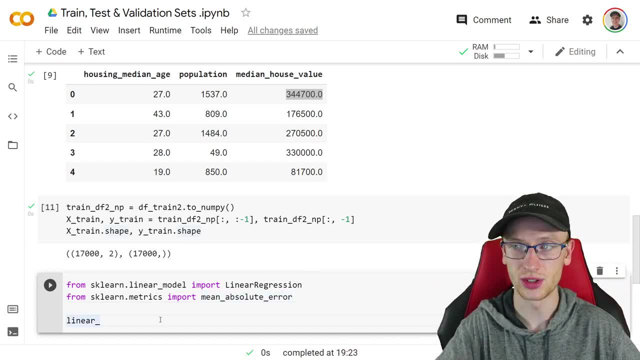 our guess or how far off is our model from the actual true answer. so we're going to fit our model or train it with. linear model is equal to this linear regression object bracket, bracket, dot fit and we just need to pass the input output pairs with x train and y train. okay, and then linear train predictions. so we're going to get the 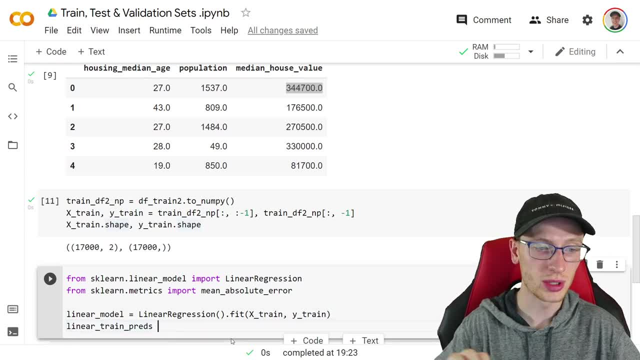 predictions for that training, this, this fit, the model. we'll get the predictions for corresponding to the inputs, and it's kind of weird because this fit probably made those. but we're just going to get the predictions again and we'll see what these are by calling linear model, that's. 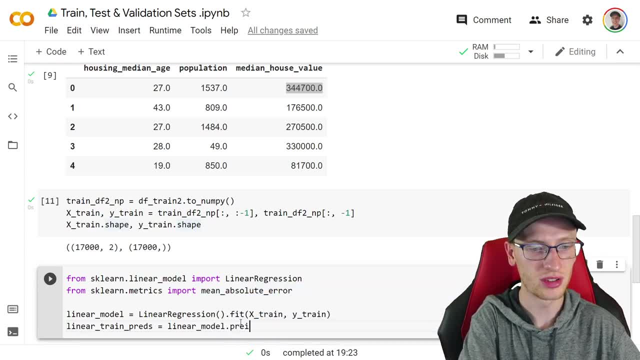 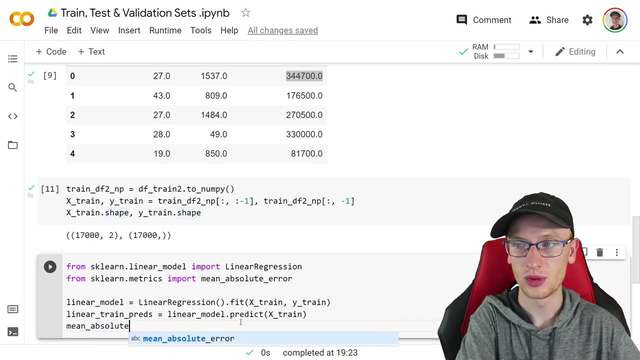 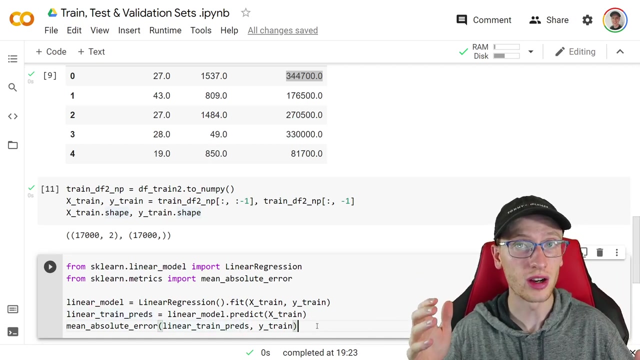 linear model model dot predict on x train. so get all of our predictions and then we can check how far our predictions are with mean absolute error comparing the linear trained threads, the predictions, to the actual training data. so this is going to show us the error on our model for the training data and we don't really care. 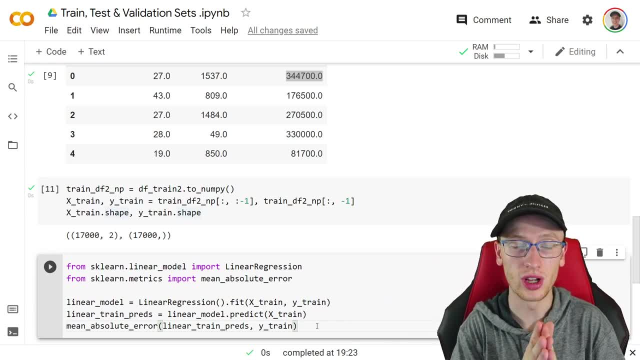 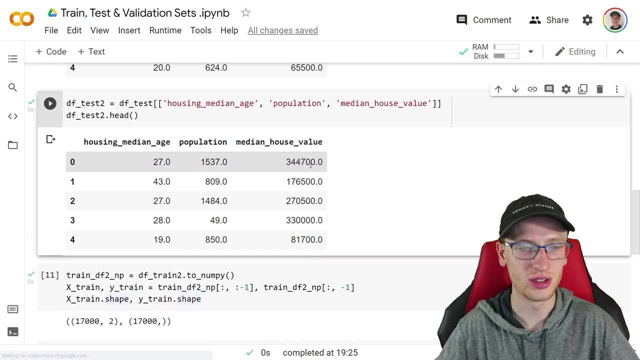 too much. we care that our model, it, can perform well on unseen data. so what we have here- sure, we have this- mean absolute error, which is 91 000 and it's- you know, it's not too bad given that these values are so big. we're off on average by 91 000 in the training set. not a big deal. 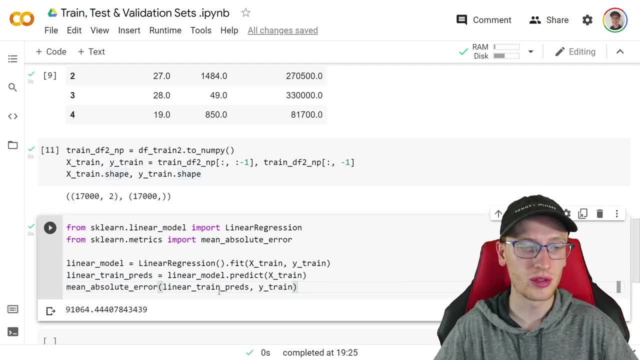 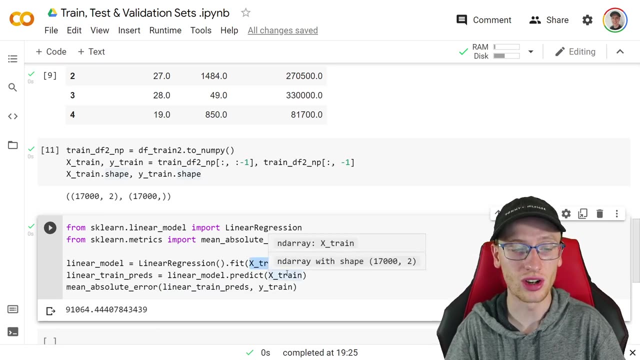 but we don't really care ever- how, at least not for machine learning type problems- about the error on the training set. we care about the error on some data set that is used that hasn't been seen before, seen being. this is seen right here. we're fitting it by training it on this data. we want to see how. 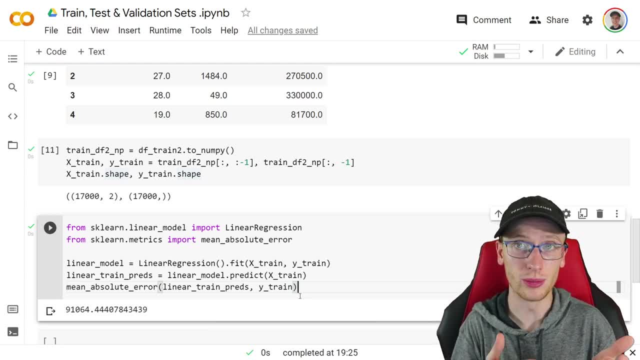 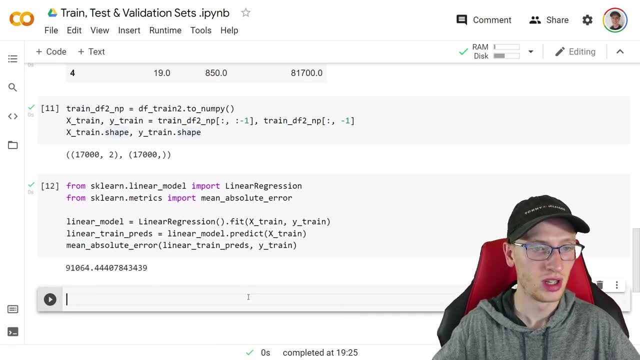 well, our model can do on unseen data, data that the model hasn't been trained with you. so to do this, okay, we have this, this test split, so we can get something very similar. it's going to look basically the same thing as this, where we can copy this and this. i believe. 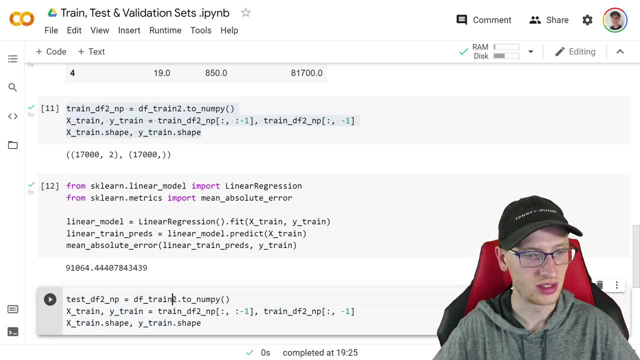 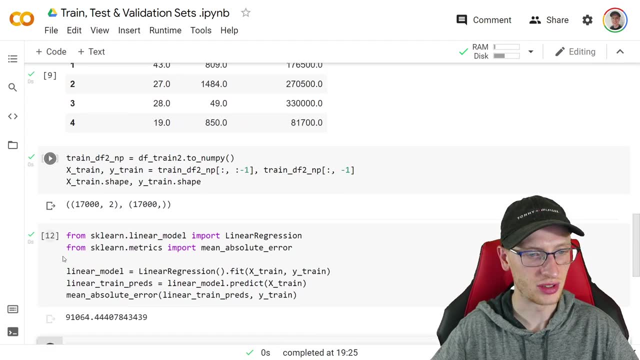 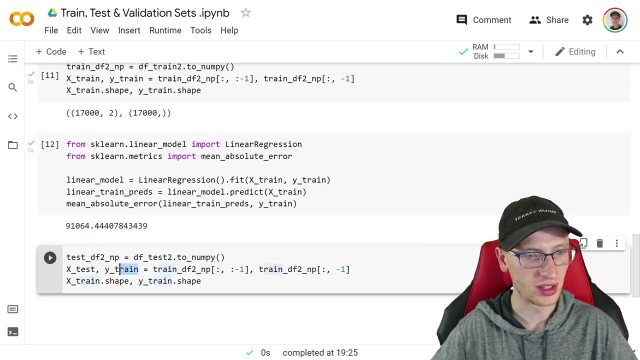 i called this test df2. numpy is df test 2, i hope, or df, df test. let me see what i called that. yep, that's df test 2 to numpy x train. this is going to be x test and y test is test and test and finally test and test. a lot of tests. okay, so that is now three thousand by two. 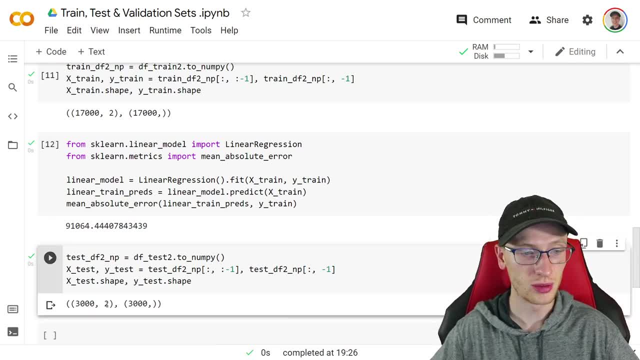 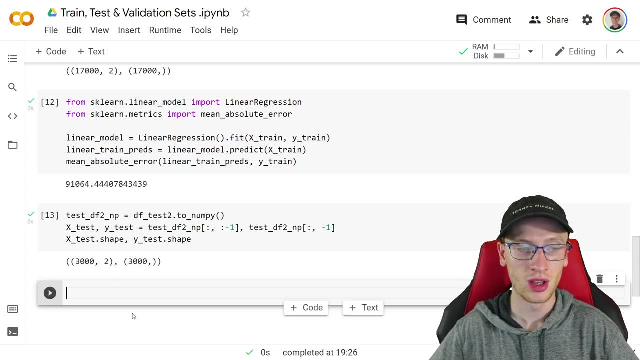 and three thousand, meaning we have three thousand rows and two columns and three thousand corresponding outputs. okay, same shapes, except we have less training examples or less less examples. so let's, let's check how well our linear model did on this test set. that's of interest to us, so let's do mean. 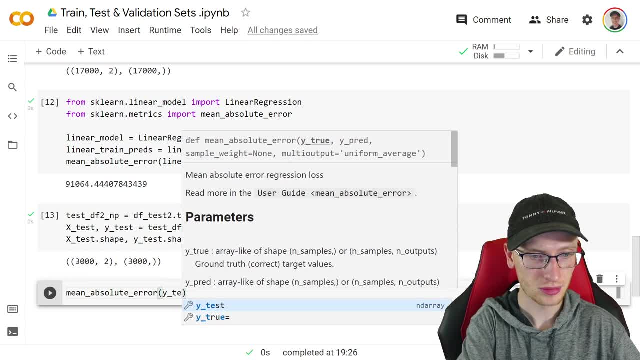 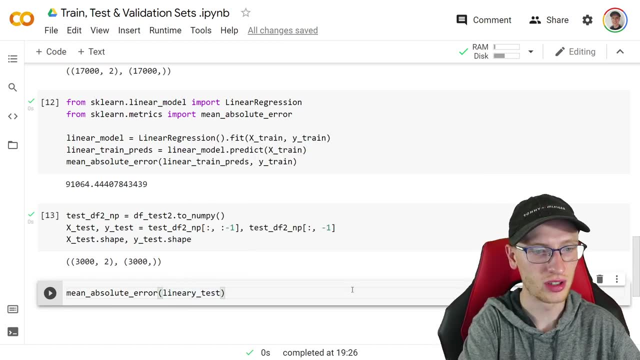 absolute error on the y test. uh, y tests. actually, i have it in a different order. i'll just try to stay consistent with the order, but it doesn't really matter. uh, with linear test, preds, which i haven't made yet, we're about to make this linear test, preds and y test and we can get this. we can. 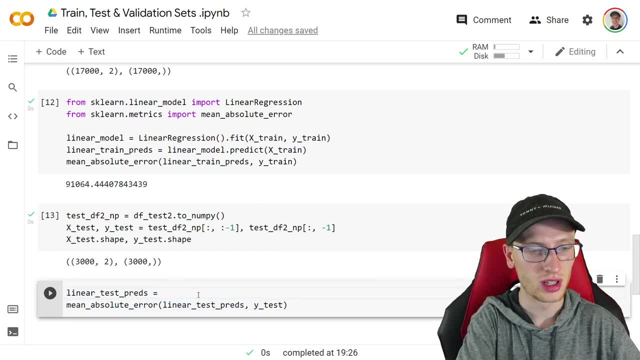 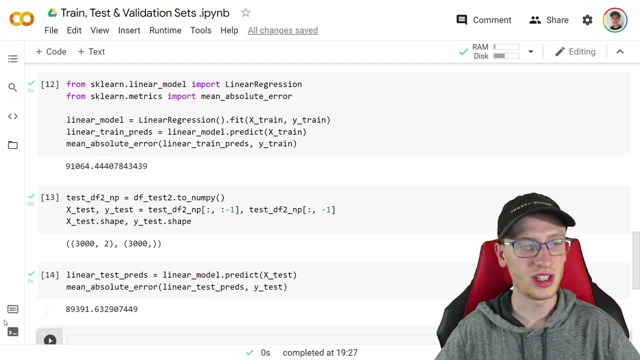 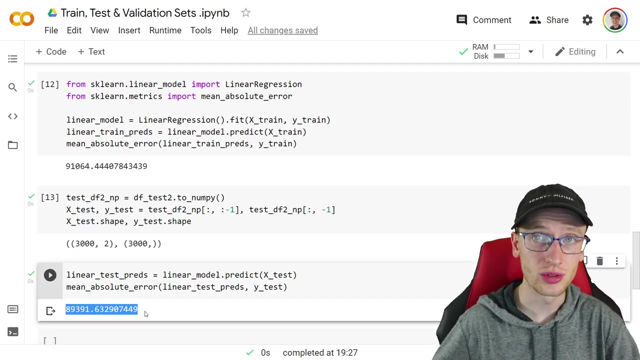 get linear test. preds is equal to linear model, dot predict on the x test. okay, and then we see this is a little bit weird to start off with because generally, uh, your error for the unseen data is generally higher. it should be higher than it was in the training set because basically your model is learning to to fit. 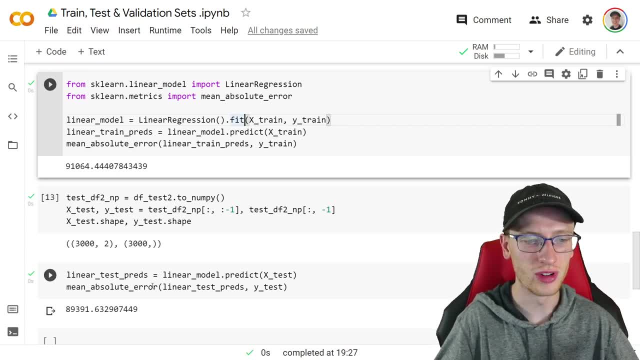 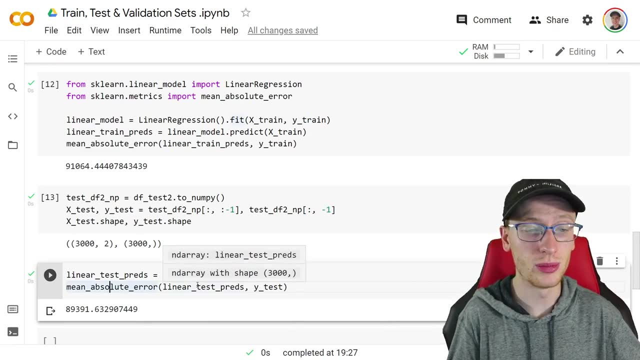 this data, on this data set, and then we check the error. it should be lower and we should have less error than we do on some data set that we haven't seen before. um, but that's what happened to be and sometimes that happens. so, anyways, we have some error here and we have some benchmark to beat. 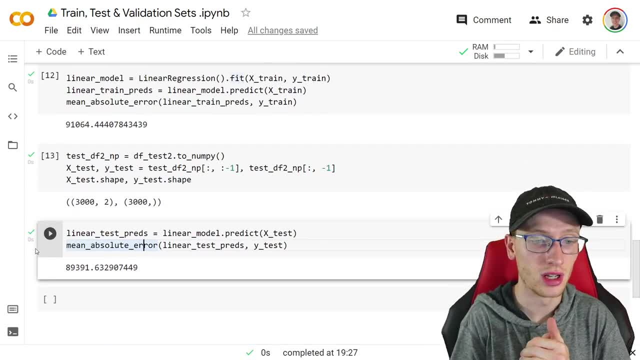 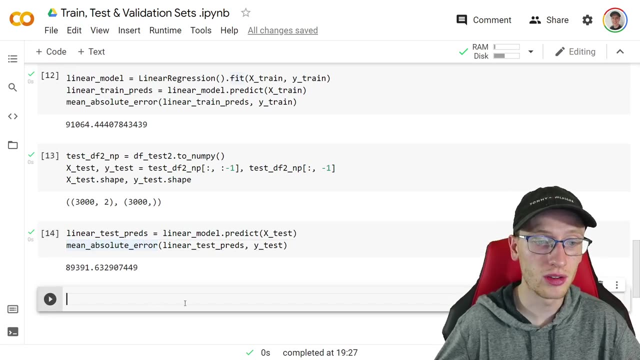 which basically, we want to train other models and see, uh, we want the best model, or i'm not going to make. show you how to make the best model, but i'll show you the process of how you would go about making the best model with this train test and validation. well, soon, validation, right now. train test idea. so if 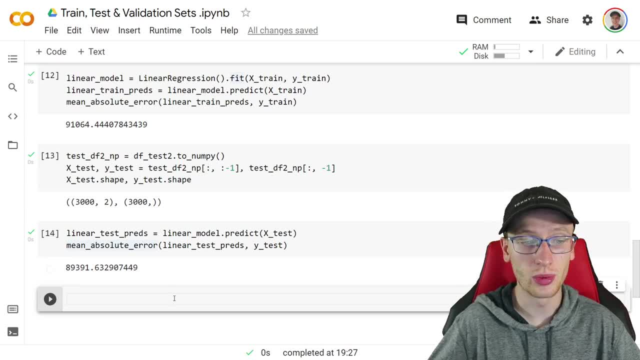 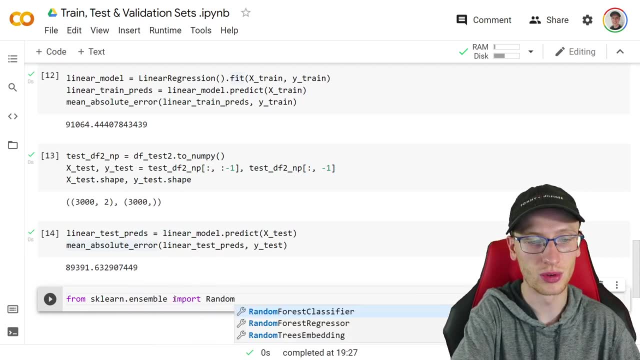 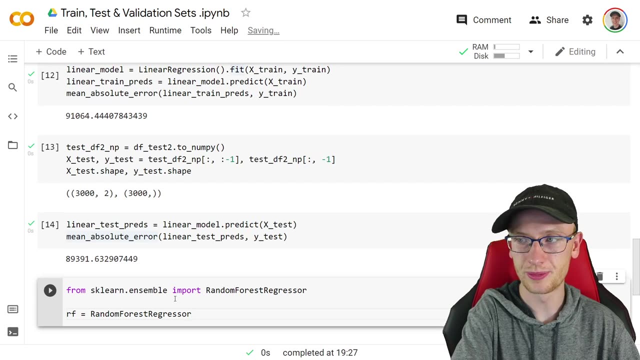 we're to make another model, let's, let's suppose we could do a random forest. so from sklearnensemble we will import random forest regressor and we'll say: rf, just our random forest variable is equal to the random forest regressor with, uh, just the default by now. if, or for now, if you guys know happen to know off by hand, uh, we can. 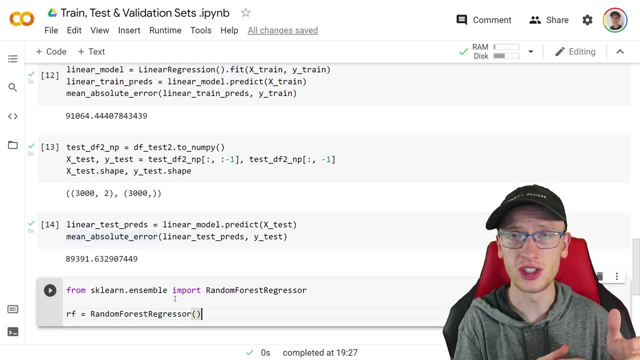 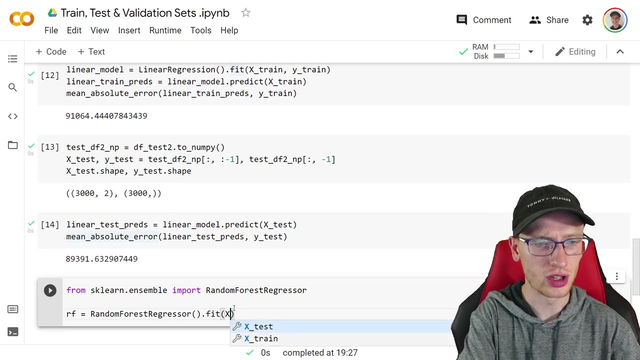 change. we can tweak this random forest by its number of trees, which is called n estimators, and it's and it's max depth, so how big these trees are basically. but we're just going to stick with the default parameters for now. we'll tweak them later and we'll do dot fit. we're going to. 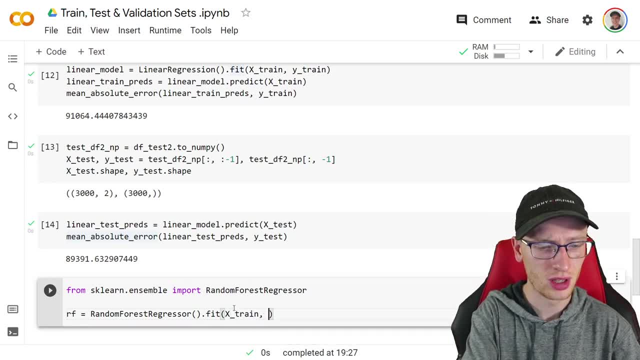 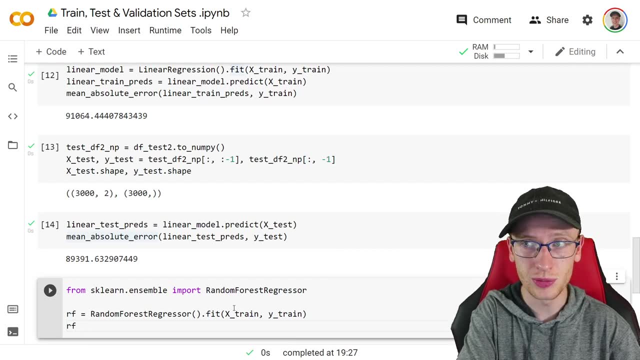 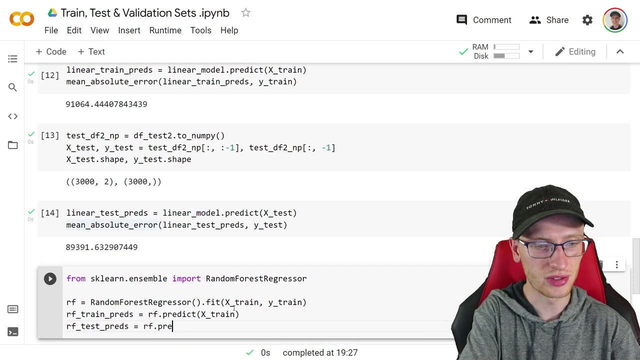 do it back same way: dot fit with xxtrain and y train okay, and then after that we can just go ahead and get the training predictions and the test predictions with rf train. uh, preds is equal to rfpredict on xtrain, as well as rf test, prez is equal to rfpredict. 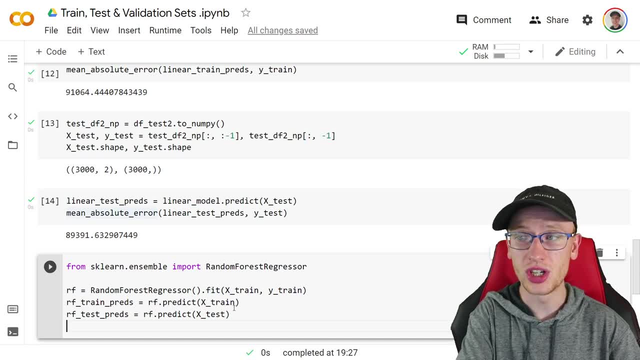 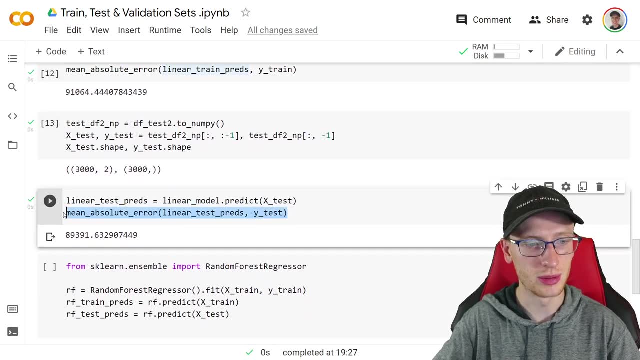 with xtest. okay, now that we have those, we can check the error. I'll just show the error before I split it out here into: here's train error, here's test error. We're going to do it both at the exact same time. 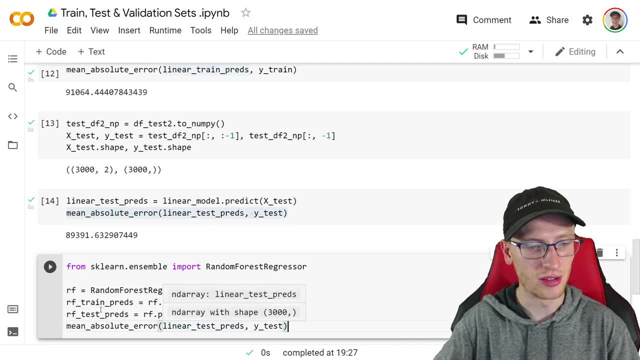 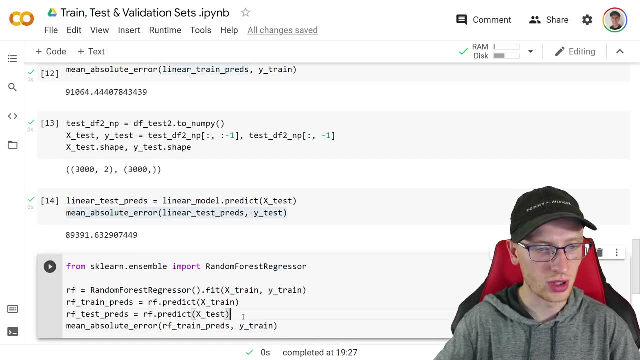 by just copying this in And we have mean absolute error on not linear test threads but RF train threads with Y train as well as the same thing. comma mean absolute error on RF test threads and Y test. Okay, so here's the error of our just base random forest on both. 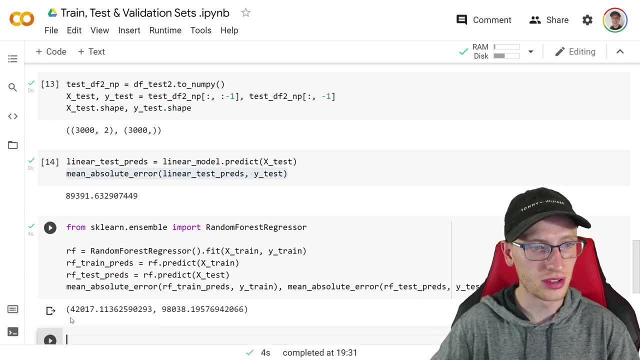 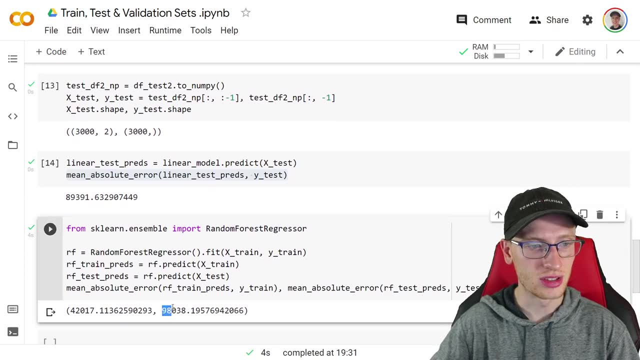 the training set and the test set It is 42,000 instead of 91,000.. That's way better, But we don't care about how it does in the training set: 98,000 on a test set compared to 89,000.. So this did. 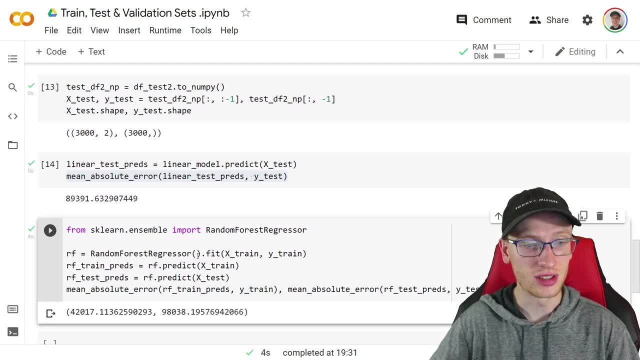 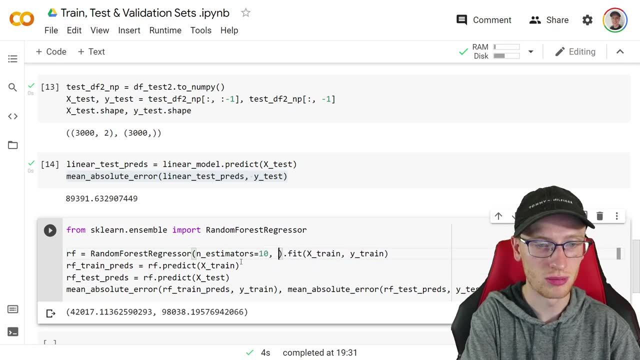 worse. Okay, we didn't like this, Let's try and tweak these things. So the way you tweak this is: I can change, say, an estimators. Maybe I can make this 10. Okay, And then I can also change max depth. I'll change that to be: 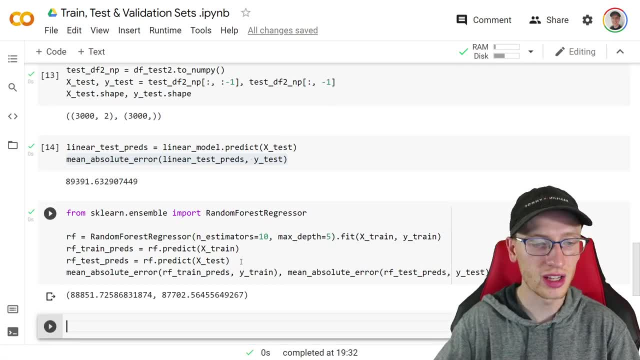 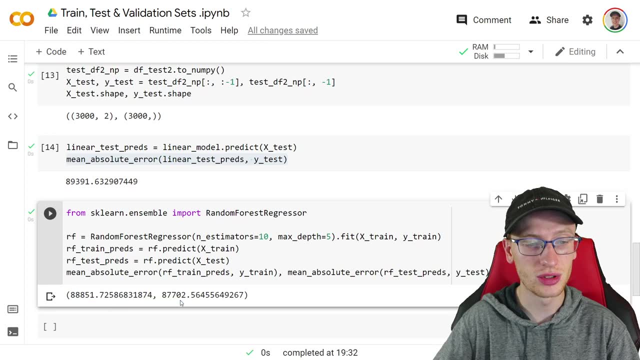 equal to maybe five, I don't know. run that again. this. I'm just going to monitor this value. For the most part it's interesting, an interesting discussion, to look at the difference between these two, But for the most part I just care about the error on this test set So 87,700. 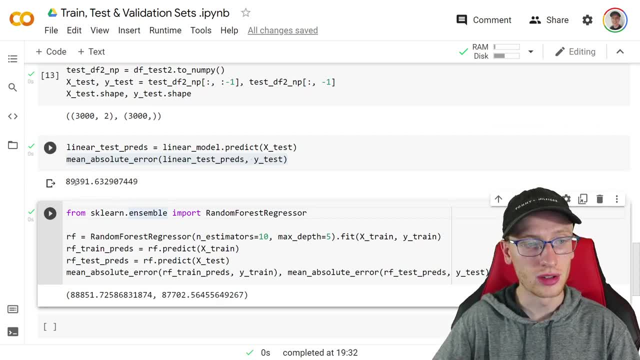 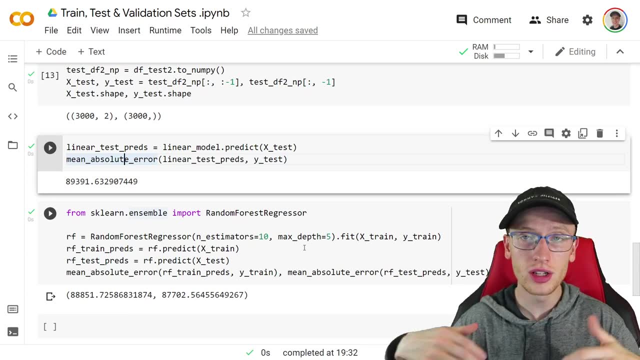 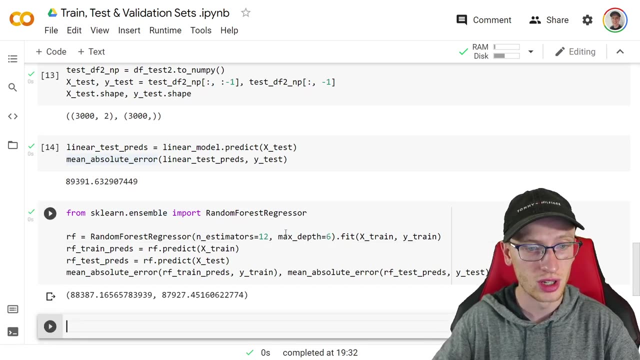 Immediately I already, just by tweaking those a bit, I got better, a lower error than the linear model did. So I played around with this and I got a better model. Now I could repeat this process and keep trying to get better and better. you know, maybe I can try 12 and six. did it? did that go down? No, it. 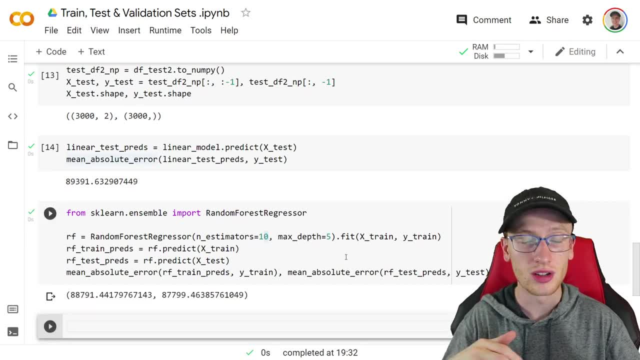 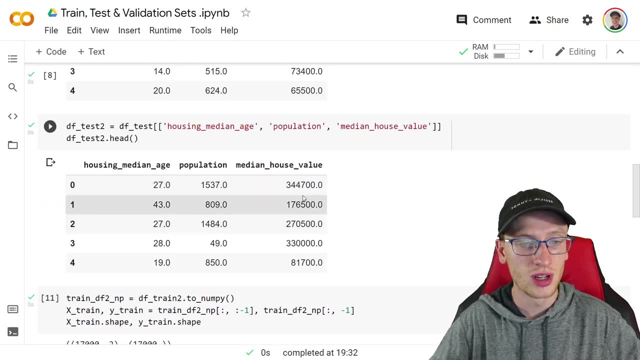 seemed to have gone up a bit, a little bit. So I'll just undo that And it no matter what I'm playing around and you can change, you could try more variables, you could do different transformations, you could play different algorithms, like a bunch of different algorithms, like gradient boosting. 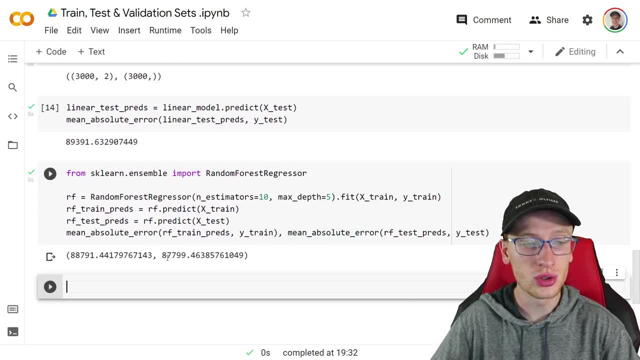 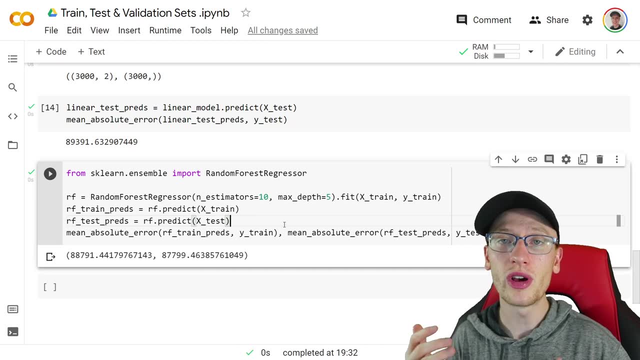 or tensor, tensorflow, neural network models- whatever you want to call it. you can change that. Now we've picked some model based off of getting the lowest test error that we could possibly get. that's great. What we want to do is now put this into production, or we're happy with our model. 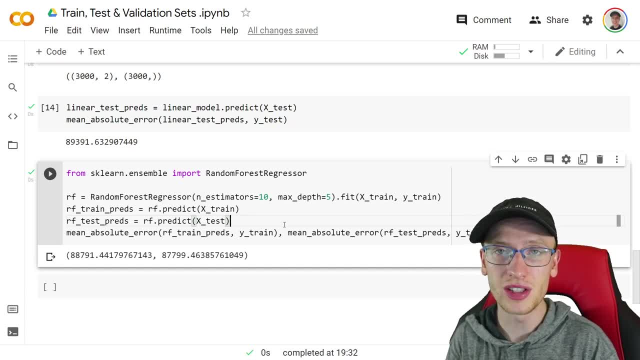 And we also want to say: hey, boss, or whoever we made this for, if it's ourselves, whatever, we want to have a valid estimate of how poorly this thing is going to do, how much error it's going to have. that's important to us. Now, what we could say is: on average, we think it's going. 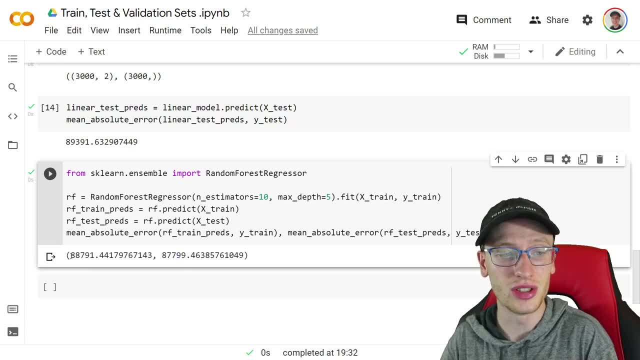 to be off by 87,799.. Or we could use this as an example. we could use this as an example. we could use this value: 88,791.. And those are reasonable estimates, but they're not nearly as good as what. 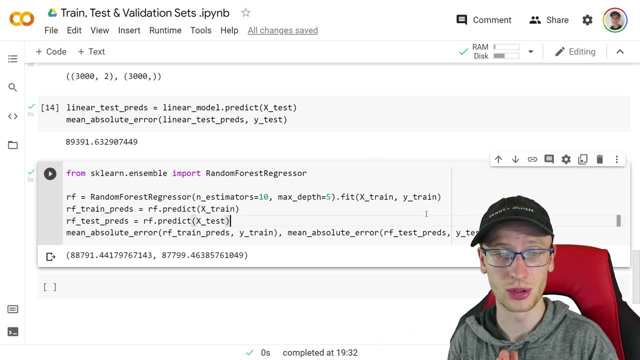 we could have gotten if we had another test data set. So basically, what we'd like to do is: have we trained this model on this data set? great, we've lowered this other error down over and over again on this, this test set here. except now what we want to do is introduce a third data. 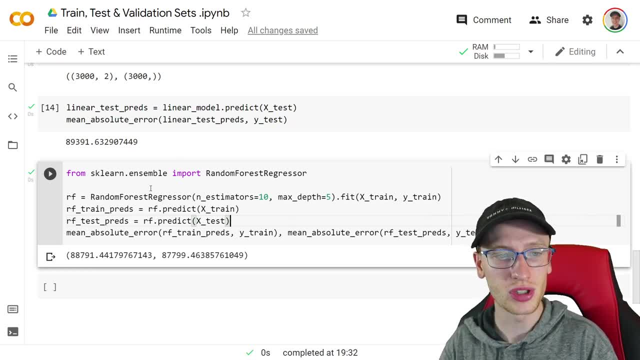 set. that hasn't been seen at all in this process. we haven't been training on it, we haven't been testing it, we haven't been testing it. And then we're going to have a separate. it has just been called, basically a holdout set, another data set, or now we can say what is actually the error of. 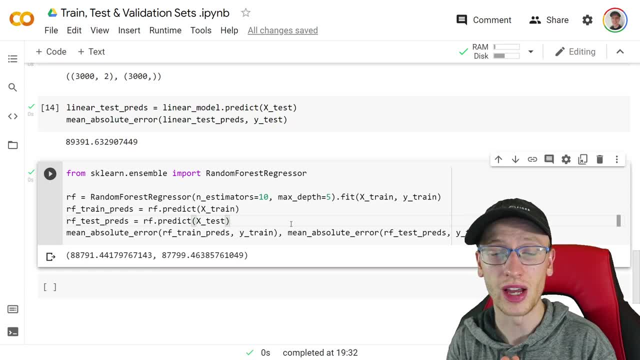 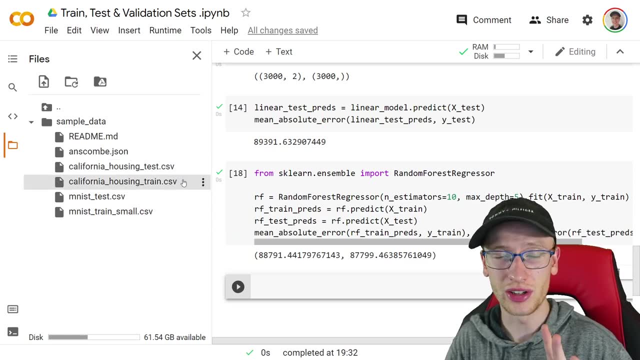 our model, And so that is the only data set that can do that accurately, And so we're going to keep that. now, generally, what you're actually given is just one big data set For us. we happen to have train and test, but that's not usually the case. Usually, you just have this big data set and it's. 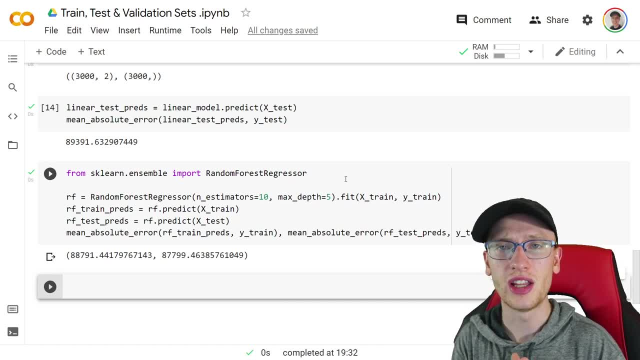 up to you to how to partition it, And so generally the split of the data is kind of, you know, shuffle it around And then you would get, say, 70% for train, 15% for validation, 15% for that final test. 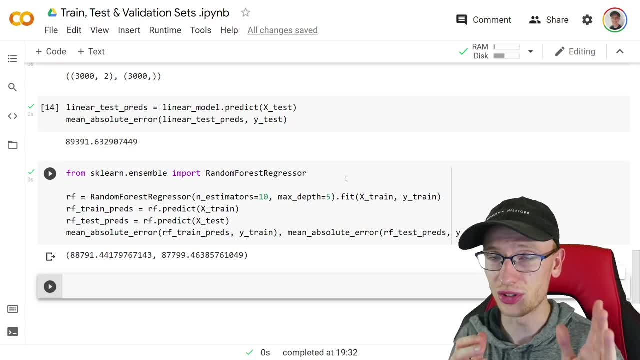 sometimes called holdout set. Validation is also sometimes called dev or development set, by the way. But I'm going to use train validation and test all the time And yeah, so that the split is up to you. But no matter what you're going to be doing, some sort of train test split function. 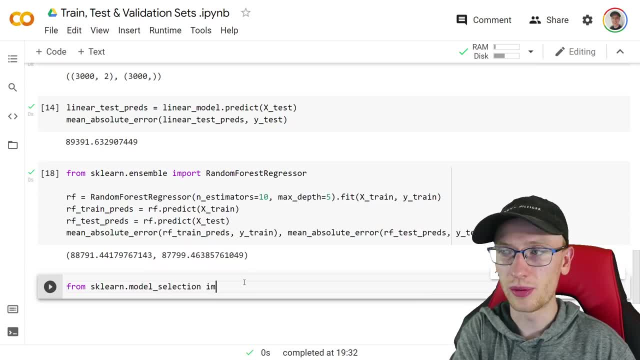 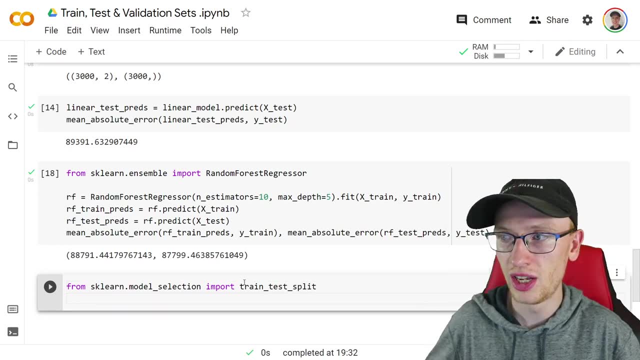 So this is called from sklearn dot model selection. we import train test split, a function that partitions both the inputs and outputs, And I'll show you how to call it like this train test splits of. we're going to give it, for us it's just, it splits whatever you give it. 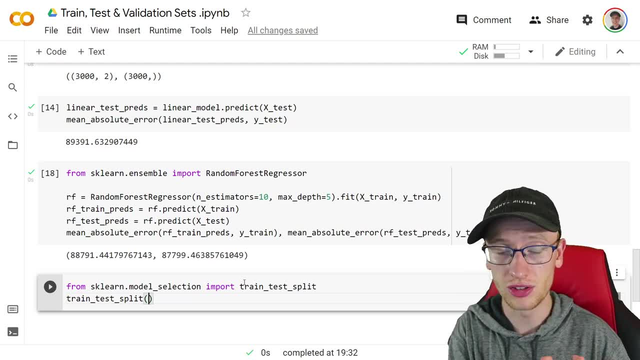 So we're going to give it tests And so we're going to split our, our test data- And I know I'm using it interchangeably, it's kind of weird, But our particular test set we're going to split that into validation and test. Okay, so train test split. we call that with x test as well as y test. 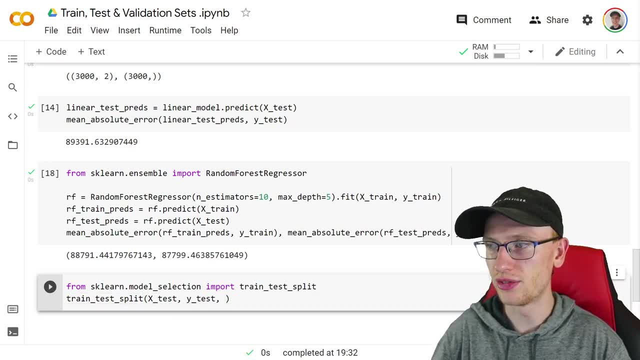 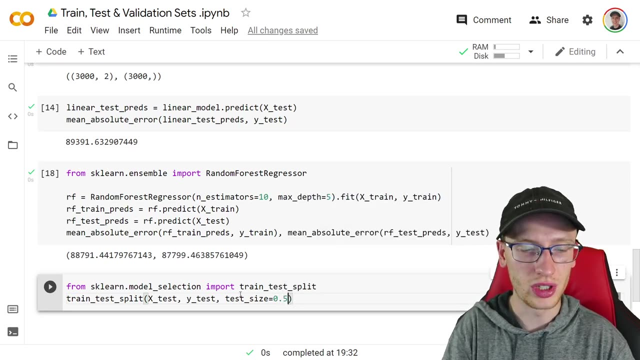 And then you can kind of specify this parameter and not just kind of you can definitely specify this parameter that says the: basically this, this split, so how much you want to split. but we're just going to do point five, So we'll do test. size is equal to 0.5.. And then what we 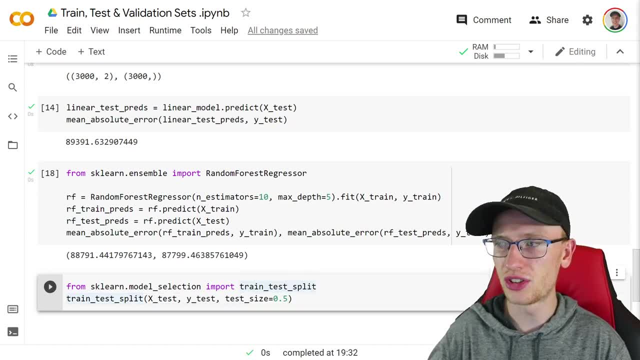 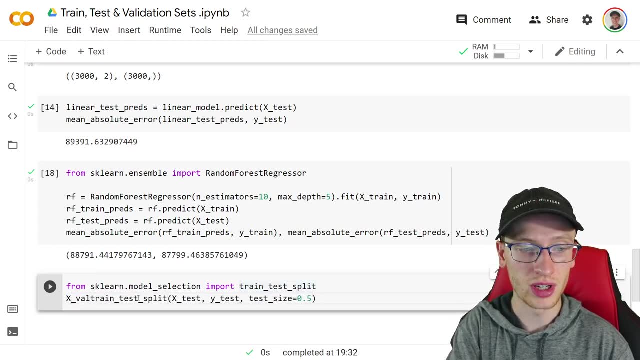 what this thing returns is. it's this organization. honestly, I always forget. sometimes I implement my own train test split function. But you can do, it's going to be x of Val for us, x of Val, and then it's going to be x. I'll call it hold out, so that are just hold, so that it's not confusing. 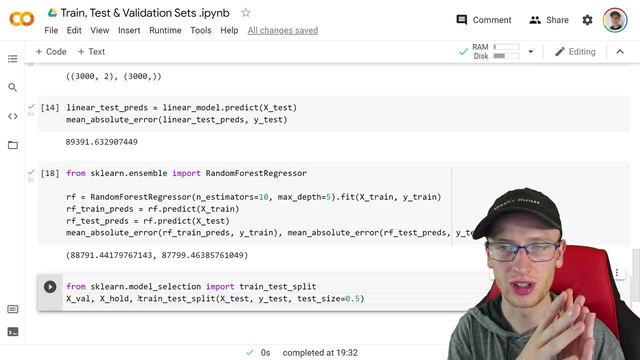 with the test, But how I was calling test before, with this third split of the data set. that's what I'm going to call here. it's called holdout because basically you, you keep it until the very very end, So x fold, And then it's going to be the y, so y Val and y hold as well, And you. 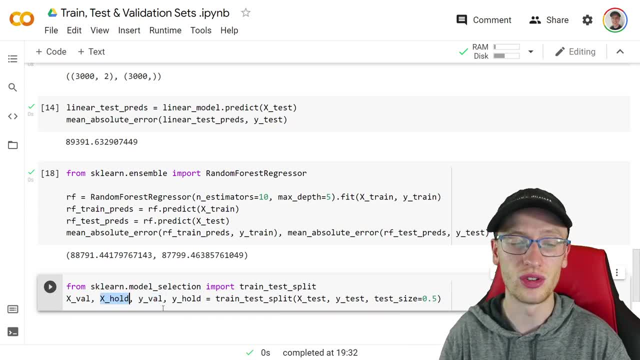 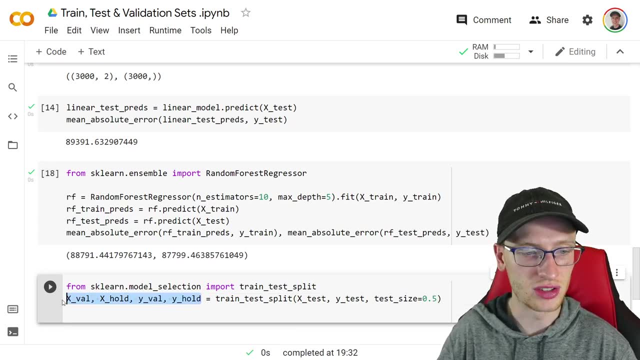 could feel free to call this test or, sorry, feel free to call hold test if you want to do instead. Okay, so we split that up And then we should see if I change this to all of its shapes. Instead we see x- Val dot shape. I'll just copy it like that: X, fellow shape, hold that shape. 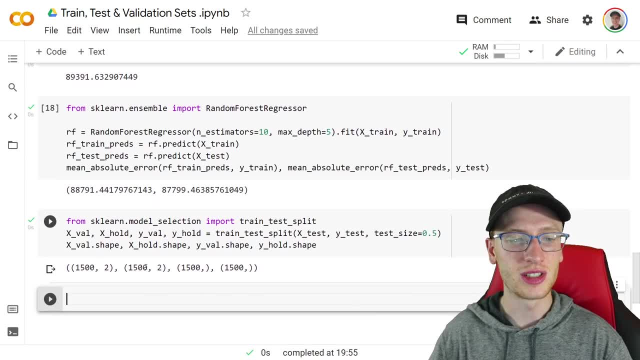 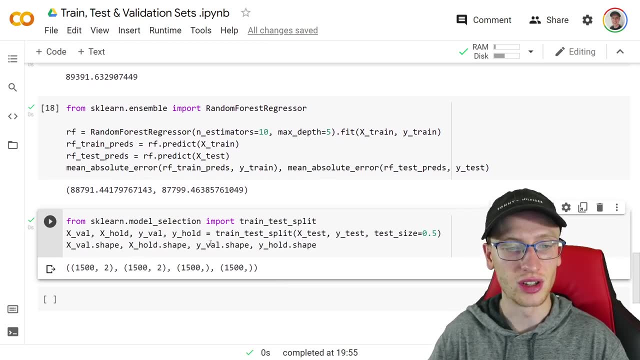 y Val dot shape and y hold that shape. we can see it split up that 3000 rows, So the 3000 by two into 1500 by two and 1500 by two, and these are 1500.. Okay, so hopefully that made sense. 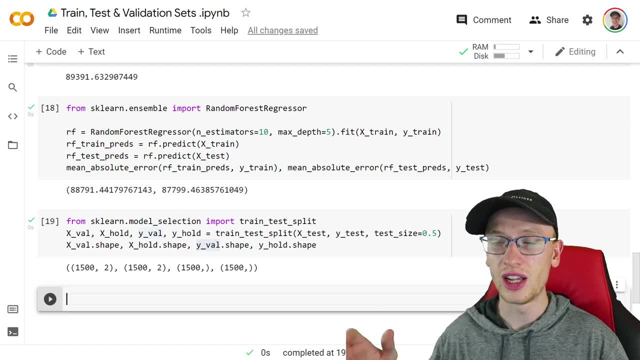 That was the the main part of this video, So I hope you enjoyed this video and I'll see you in the next one. Bye, understand that for sure. And now just to show you how you do it, To finish off our project here. 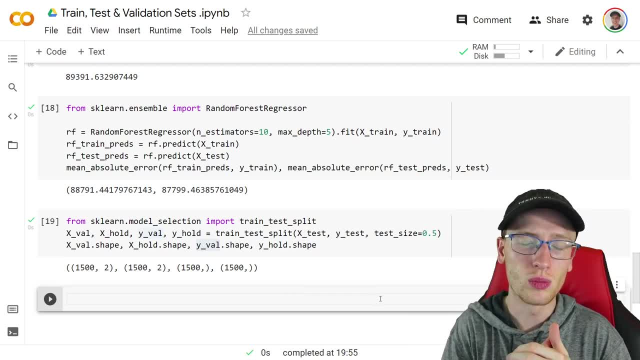 we would get some, so maybe okay. so what we would have done from the beginning is train models on the training sets and then evaluate their performance on the validation set, try to lower that, and then we pick one and say: actually check its error on the test set. So let's do that. 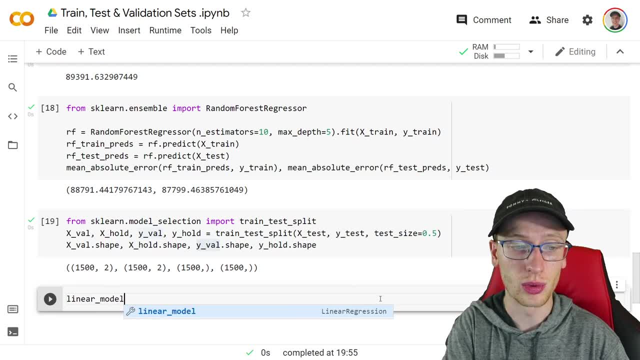 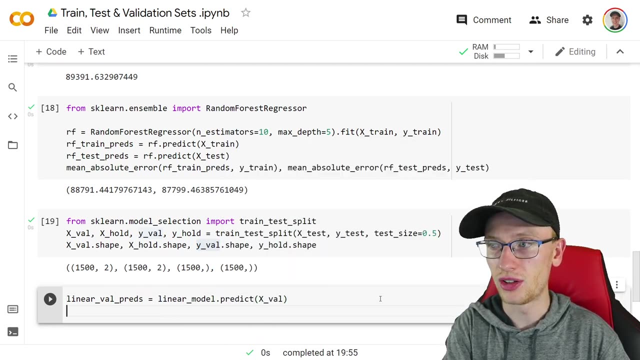 quickly, We've already trained the models, So we're very happy. We're fine with the trained models here. So what we can do is get linear validation predictions. is linear model when your model dot predict on x Val, okay, And I can get the error on the training set as well as the validation. 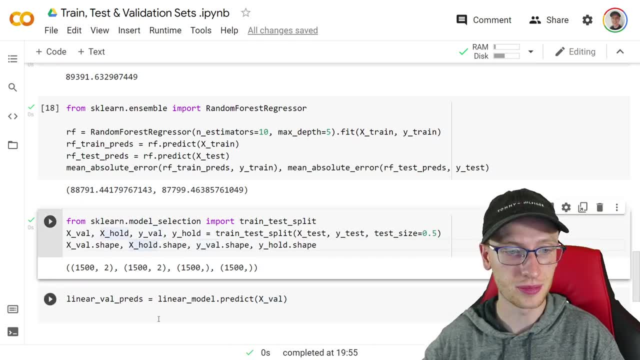 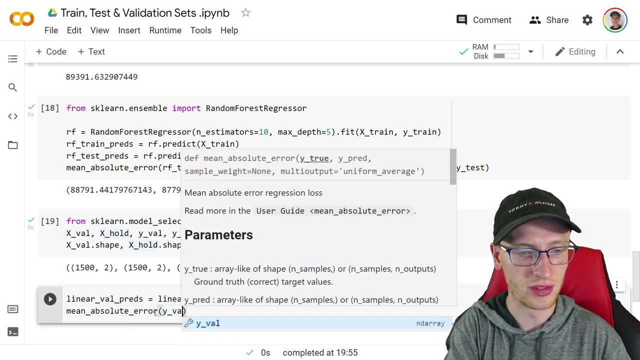 I'm not going to look at the error on the test set quite yet or the holdout set, But I'm going to say mean absolute error on it's going to be. I'll pass it: y Val as well as linear Val friends. 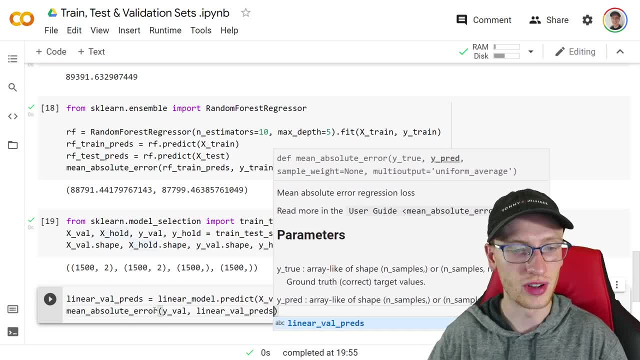 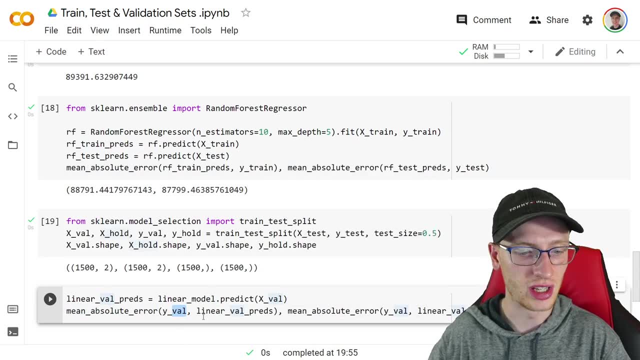 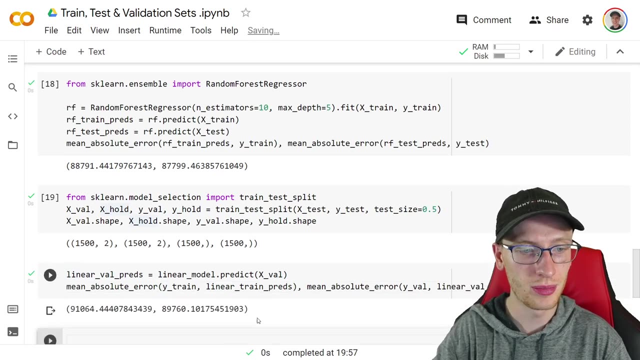 okay, so that's going to be on the validation, And I guess I'll look at it on the test set as well. So the second one will be validation. This again, I will say: we've already looked at this value. this should be exactly the same, But I just want to show it as well. Okay, so we make a. 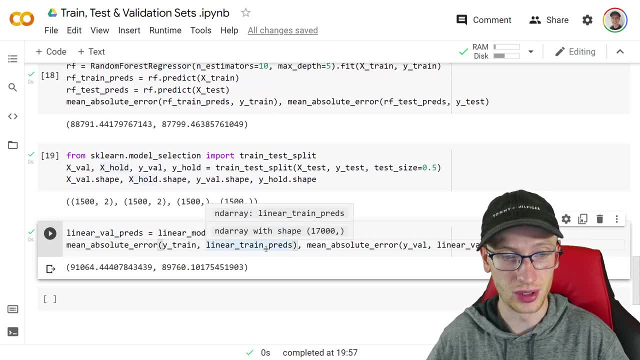 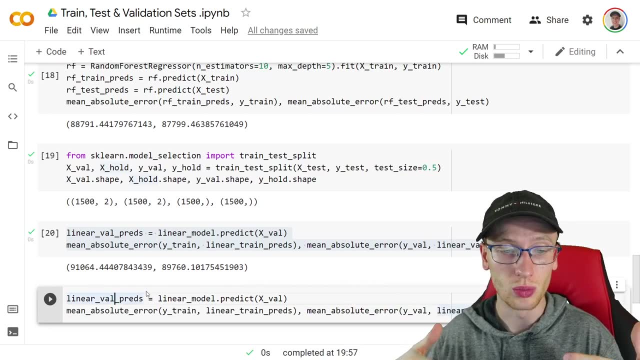 linear model. This is how well it did on the validation accuracy- Interesting. Now let's copy this and then make it for the random forest model And, if you want again, we're basically saying we're starting from scratch here. Yeah, we are training, we are using the same trained. 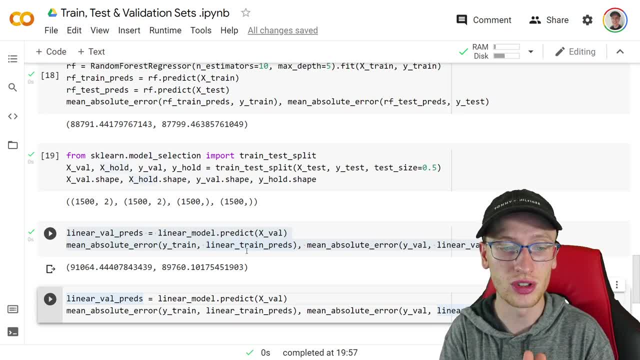 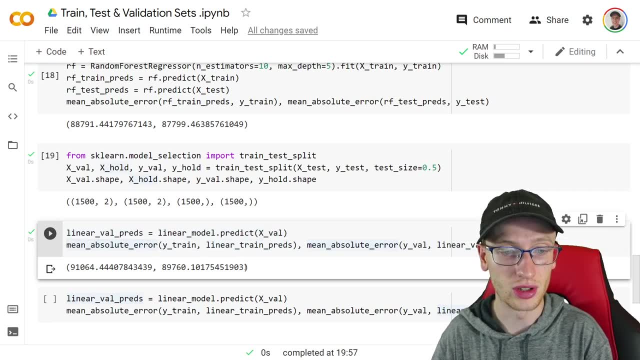 models. But I'm saying that if you were to actually do what you were supposed to do, go ahead and make whatever kind of models that you want to right now and sit here comparing the, the validation accuracy, we get an error. we want us to get the lowest of this, no matter what. 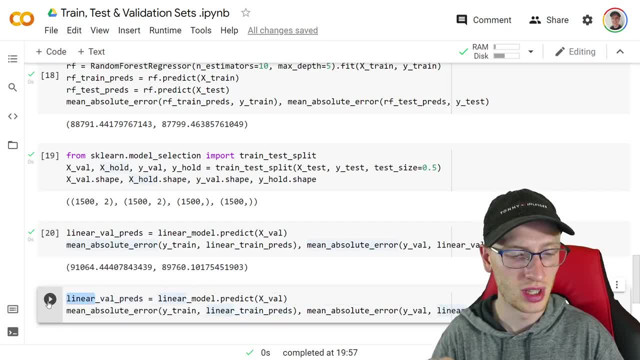 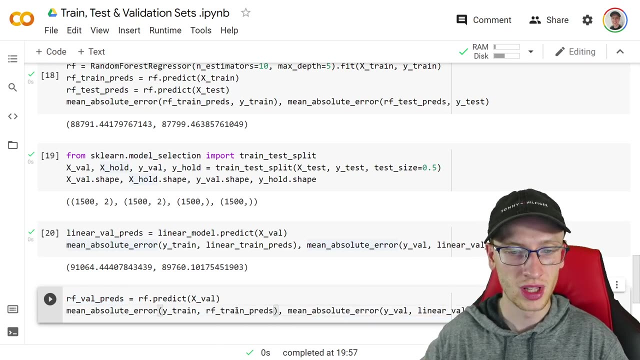 So linear Val is going to be converted to this is going to be RF Val Preds And this will be rf dot predict on x Val. that stays the same. Get the y train And when you're sorry, this will be converted to rf train Preds And this last one will be: 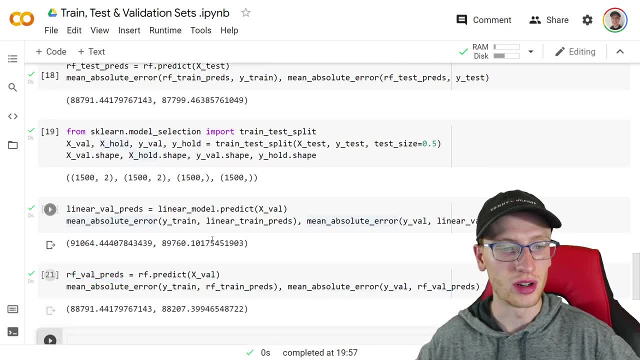 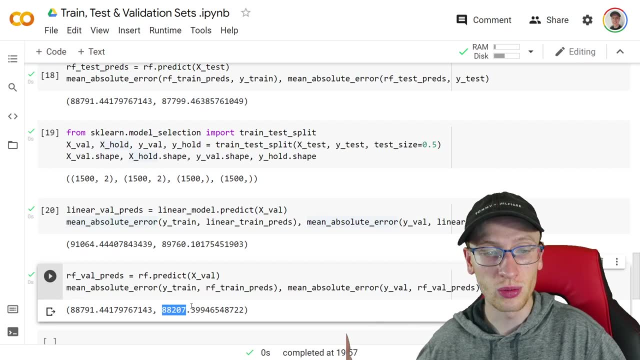 rf: Val Preds. Okay, so here we have an error of 88,000 on the validation set. Okay, so it is lower. we could do whatever we wanted to try and get this, get this to be lower. we pick a model. the model that we're happy to be picking is just for simplicity. 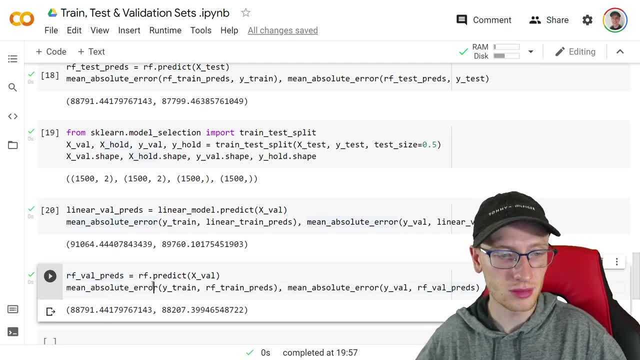 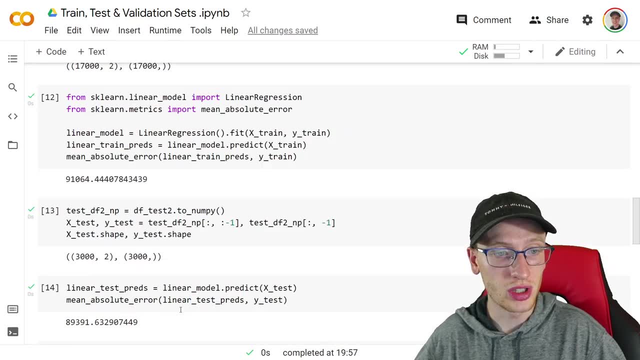 going to be the same random forest. it had the lowest validation, Okay. and now actually just to really prove that point of what we're trying to do here, we got 88,207.. Let's quickly try to beat it. And so if we go up here to sorry for the headache. 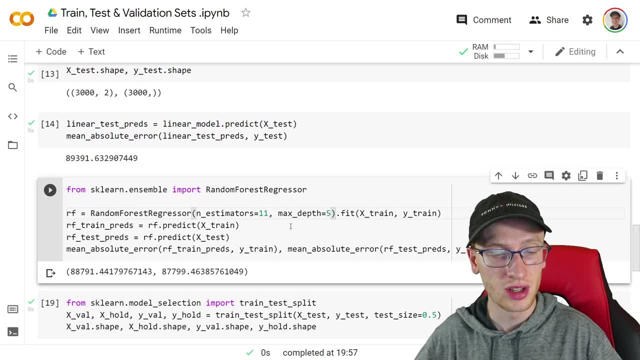 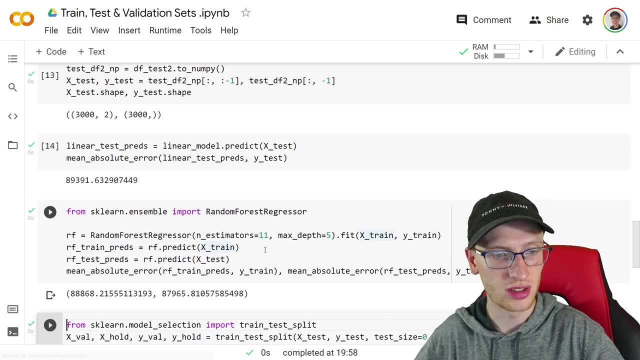 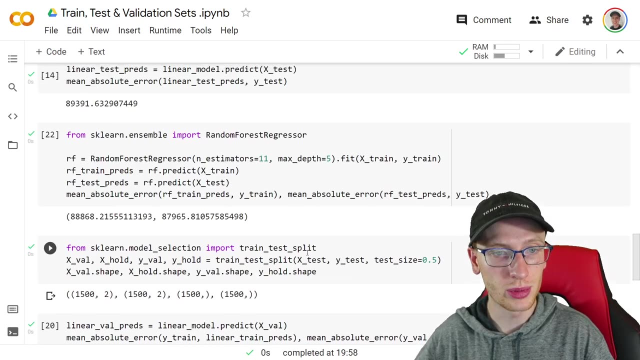 maybe we go to this: okay, change this to 11.. And just for fun. So here we are trying to beat 80,207.. And here we get- if I train that, don't worry about these measurements- right here: 80,207.. This error went up. okay, we weren't as happy with that. we're going to stick with that. 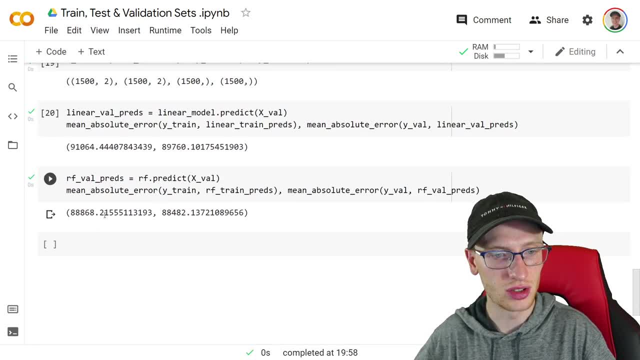 other parameter Of 10.. And don't worry about that, It goes back to what it was before. Sure, we're happy with this, we'll pick that model. So now we've picked a model, we are just going to look at the test. 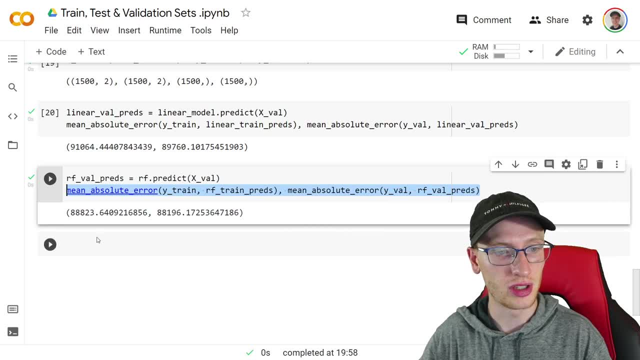 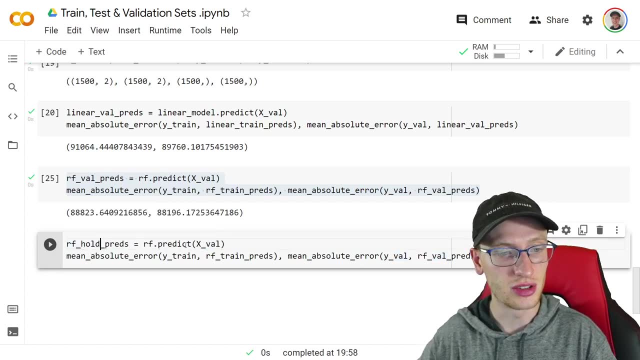 or holdout error for our final model here. So we're going to copy basically this whole thing here. we're going to say RF, I'll say hold or test Preds, RF holdout Preds is going to be this: RF dot predict on x, hold that third split of the data and then mean absolute error on y test. 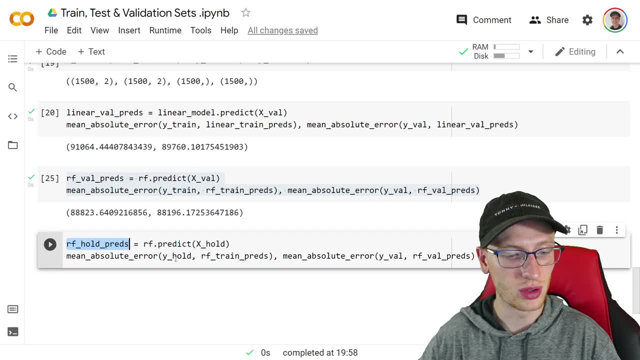 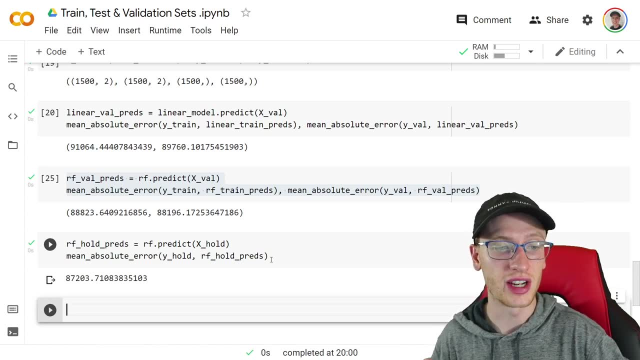 Except actually y hold. So on y hold and then RF holdout predictions like that, And we can see that the error we can report back and say, Hey, our error is actually 87,000.. Now, and I know it's kind of weird that before I said this was probably overly optimistic.